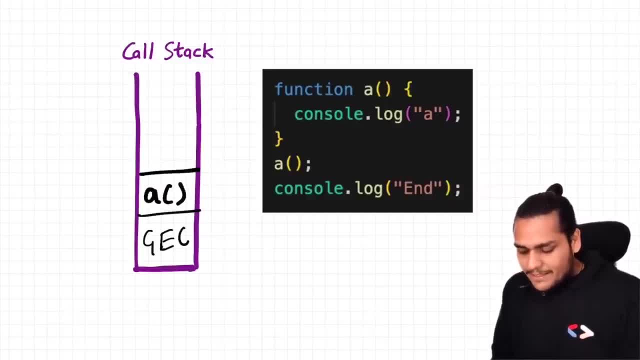 so now a will be inside the call stack. so over here now the code of this a function will be executed line by line. so this code will be executed line by line. so that means it will print a into the console. so we don't have a console right now, let's create one. 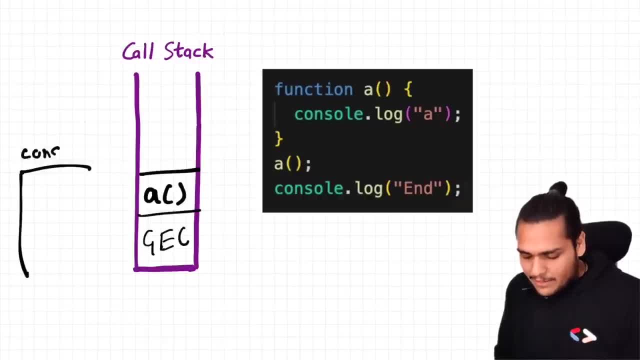 console. so we have- suppose this is our console, let's name it console. so a will be printed inside this console. so now it moves to this line. it sees that there is nothing more to execute inside a, so it kind of pops off this a execution context out of this call stack. 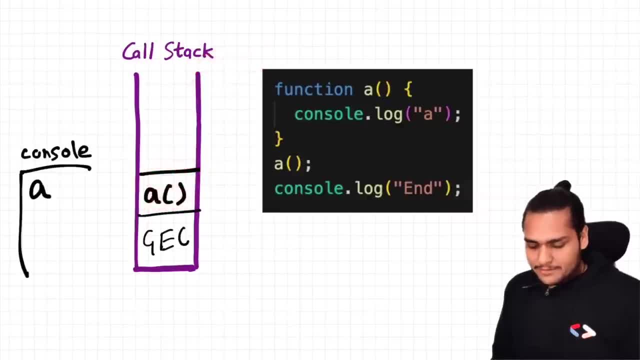 okay. so now this a's execution context is just gone. it's deleted, right, so let me just remove it. so now the control moves on to this line. it executes console log end and it prints end into the console. let's do that. so now end is inside the console. 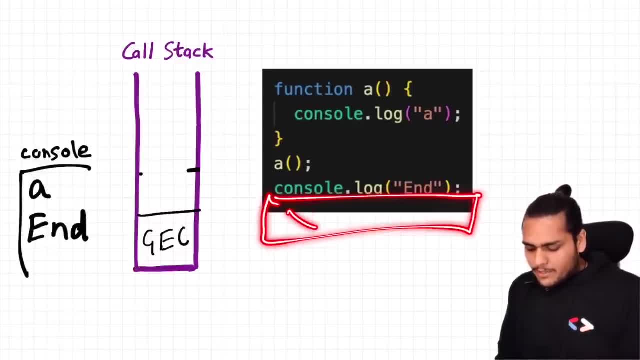 right after executing this line, there is nothing more to execute. that means we don't have anything else. now our global execution context also just pops off the call stack. we are done with running our code. so that's how the whole javascript engine executes her whole javascript program. 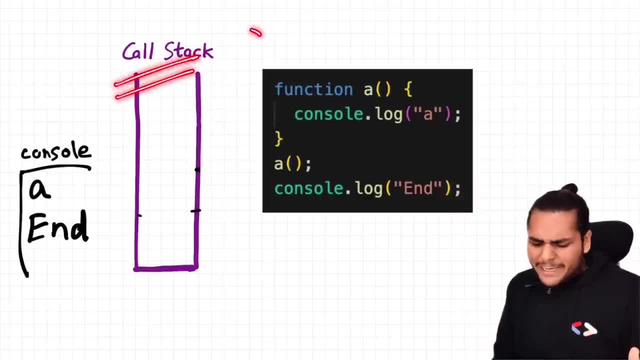 that's how it is. so the main job of this call stack is to execute whatever comes inside it. that's all it does. it does not wait for anything. if you give it anything, it just quickly executes. that that's how it works. so that is why i also say that time tied in javascript. 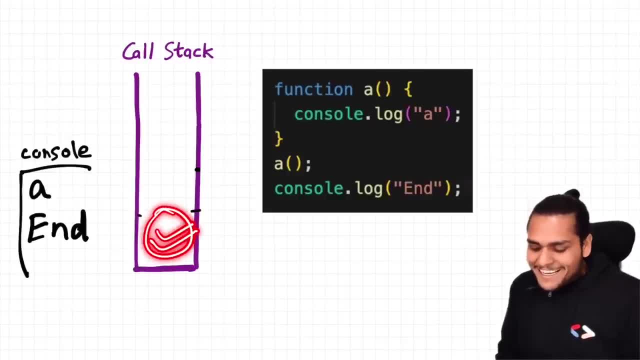 waits for none, because all javascript code is executed over here and this call stack won't wait for anything. if anything comes inside this call stack, it quickly executes. that's how it works, but hold on. what if we need to wait for something? what if we have a program or a script which needs 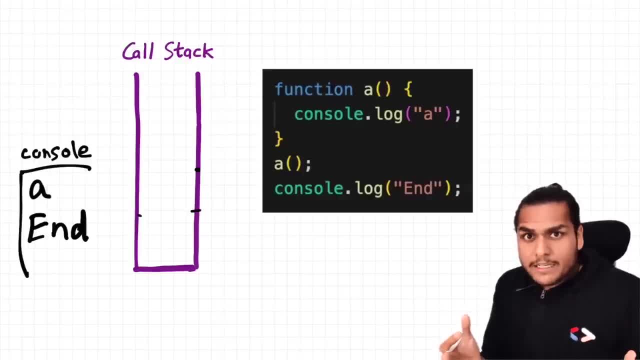 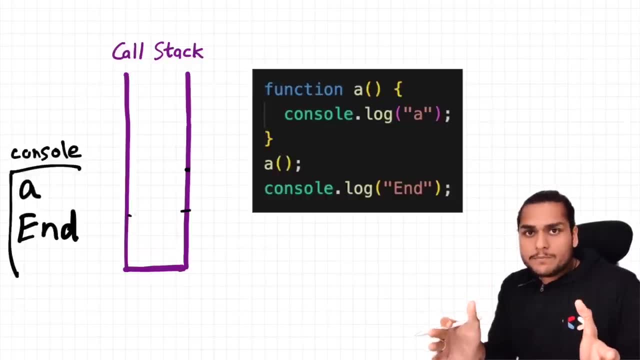 to be run after five seconds. can we do that? no, we cannot do that, because whatever comes inside the call stack is automatically quickly executed if you give it a script and say that, okay, execute it five seconds later. it cannot do that because it does not have a timer right. 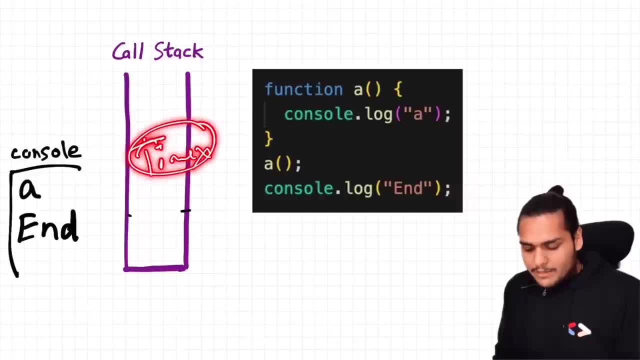 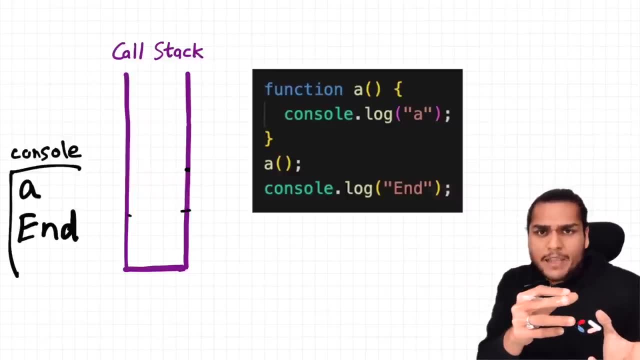 this call stack does not have a timer. so suppose if we have to keep that track of time and we have to execute some piece of code after certain delay, we will need some extra superpowers, that super powers of timers. so let us now see that how we can get the super. 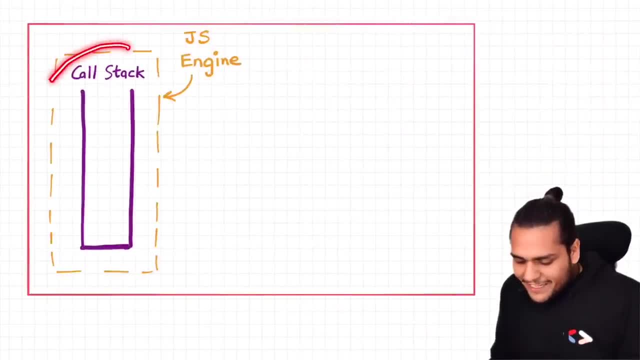 power. so this call stack, what you see over here, is inside the javascript engine. okay, this call stack is inside this javascript engine and this javascript engine is inside a big red box, right? what is this red box? can you guess it? Yes, it is the browser. okay, 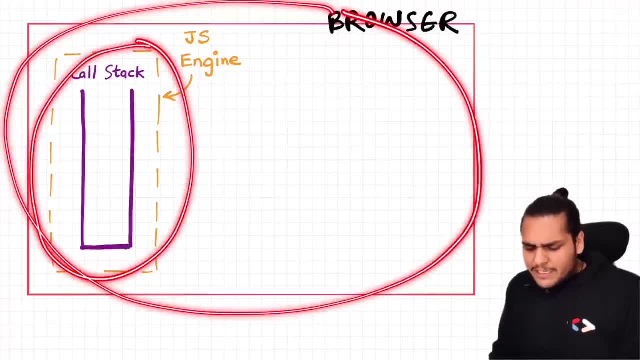 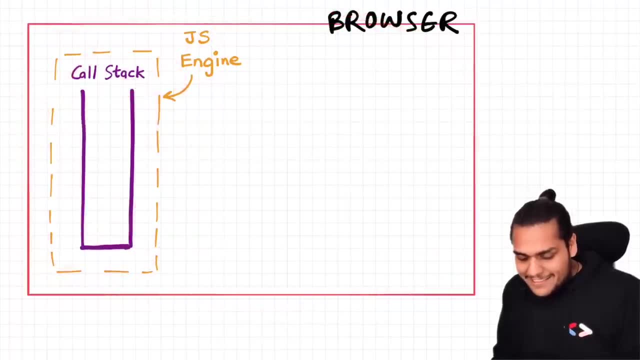 So this browser overall has JavaScript engine in it and this JavaScript engine has a call stack and over here our program runs right. This is the actual place where JavaScript code executes right. So this browser over here is one of the most remarkable creation in the history of mankind. 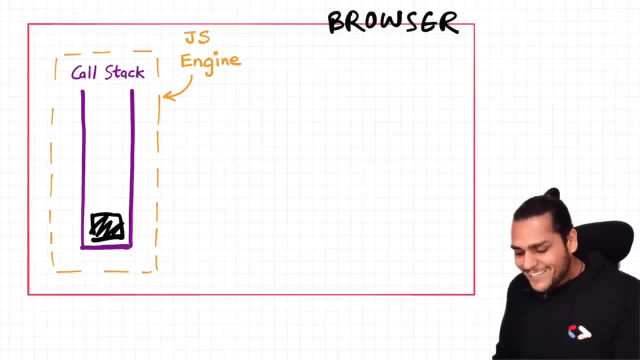 isn't it? If you don't trust me, let me show it to you. So this browser has the JS engine inside it right? And it also has something known as local storage- right. It can store some data inside it, right. 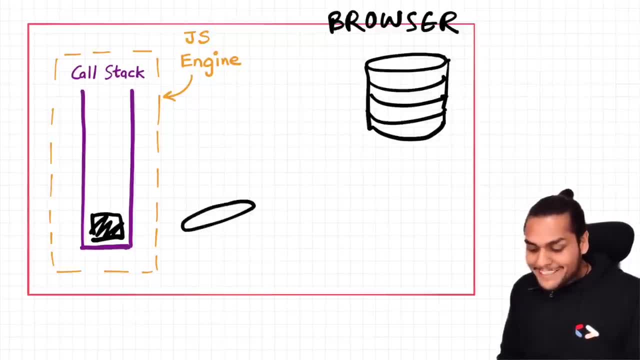 You can do that inside browser. You can also have a timer inside a browser. okay, Browser is super powerful. You can have a timer inside the browser. You also have that URL right Where you write netflixcom and so on. 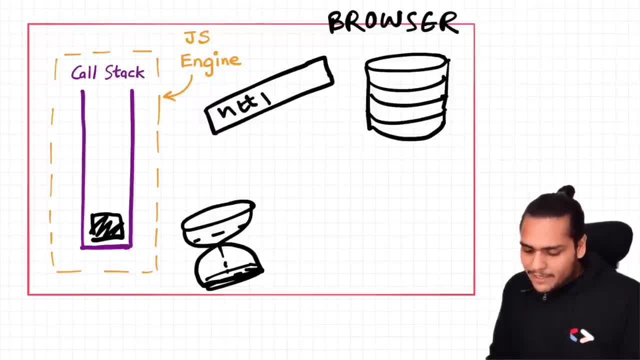 You can go and access your best TV series. this URL HTTPS isn't it- And TV series right. So this browser has this super power of communicating to the external world right Like the Netflix servers. So suppose if we have this Netflix servers over here to fetch our best TV series right. 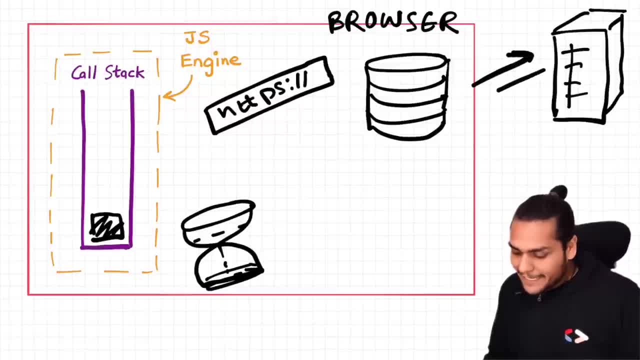 This browser can make connection to these servers, isn't it? And get data over here, And even after that, you can also have a TV series, Right? And even after getting that data, it can also display it onto the UI. Remember the browser which we see on our screens, right? 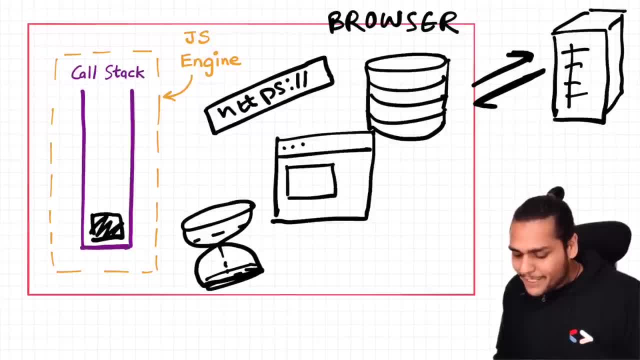 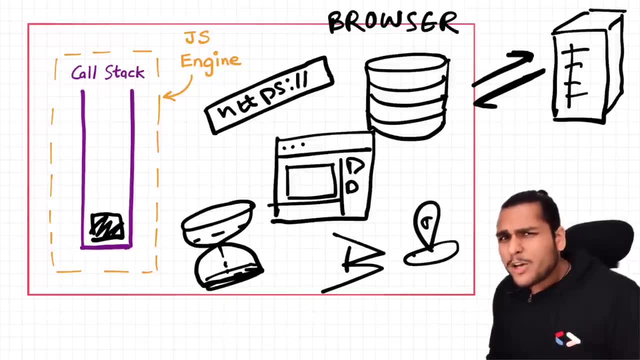 That cute little browser over here which displays the video and shows the suggestions and does a lot of things. And not just this: it has access to various other superpowers like Bluetooth access and the geolocation access and a lot of other stuff. So do you now believe me that it is one of the most remarkable creations in this world? 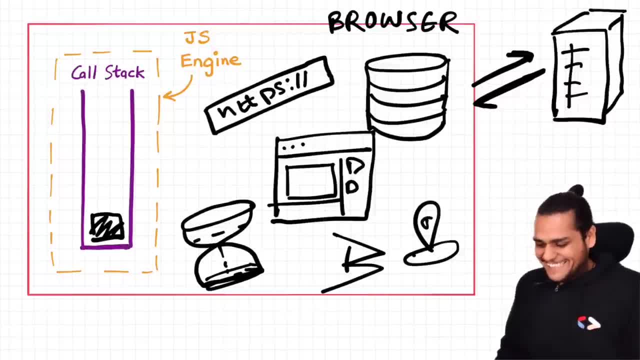 the history of mankind, isn't it? you can do a lot of stuff, right? so now, suppose, in a javascript code which is running over here, inside this call stack, we need access to these superpowers of the browser, right? suppose if we need access to this timer. suppose if we need access to this page which? 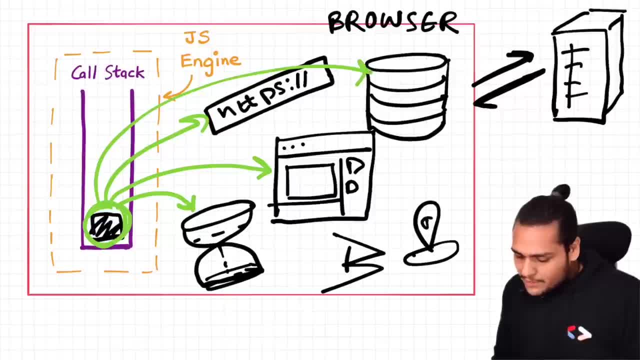 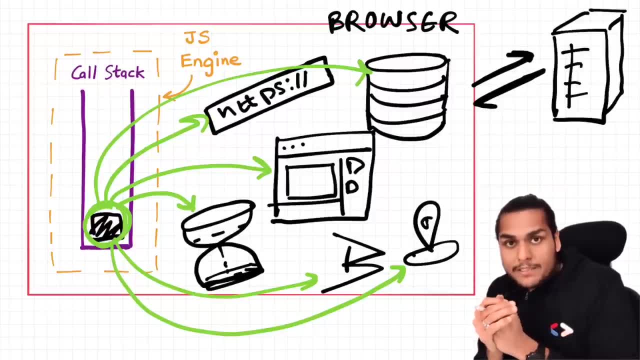 is being rendered, or the url, or the local storage or or the bluetooth or whatever, like all these superpowers. right? if we need access to the superpowers, we need to have that kind of a connection. right? this js engine needs some way to access those superpowers. right, let us see how we 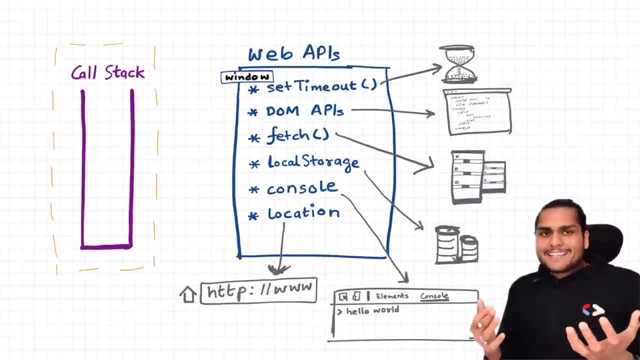 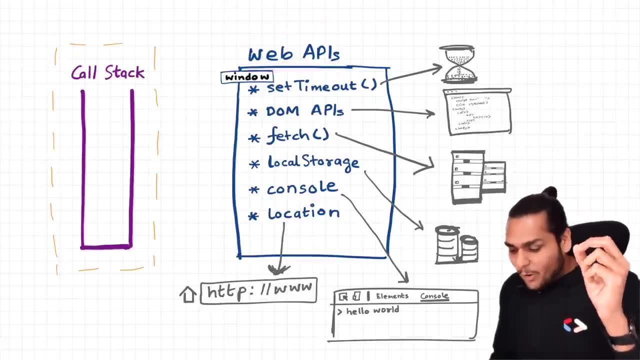 can do that. so, as we move on to the next slide, with a big round of applause, let us welcome the web apis. yes, so to access all those superpowers, we need web apis. okay, let's see what are some of these web apis. okay, so we have this web api set timeout. you know it will be a heartbreak. 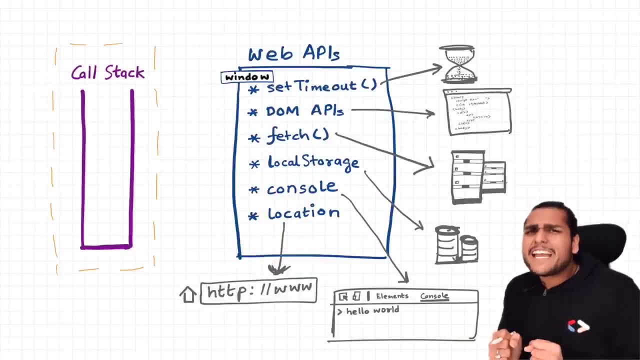 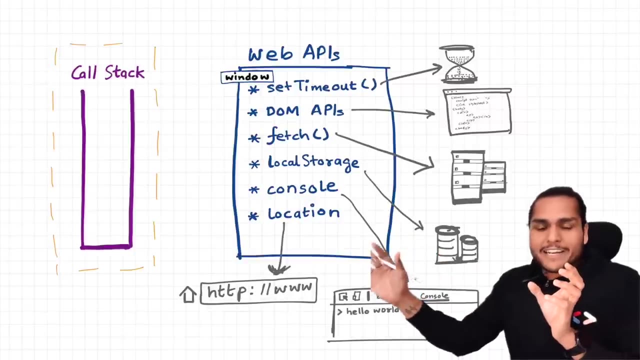 to a lot of js developers if i tell you right now that set timeout is not a part of javascript. yes, i repeat, set timeout is not a part of javascript. even the dome apis, right, the document dot, whatever you do, document dot, get element id, or whatever you do- is not a part of java. 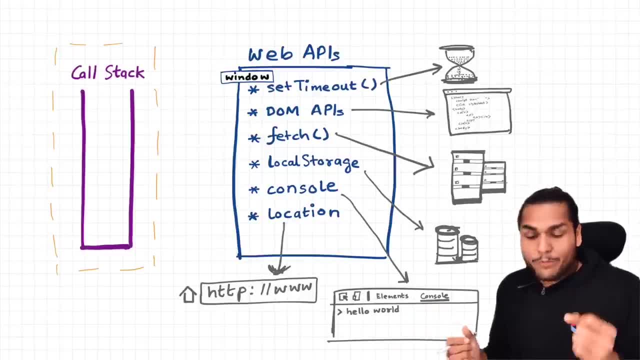 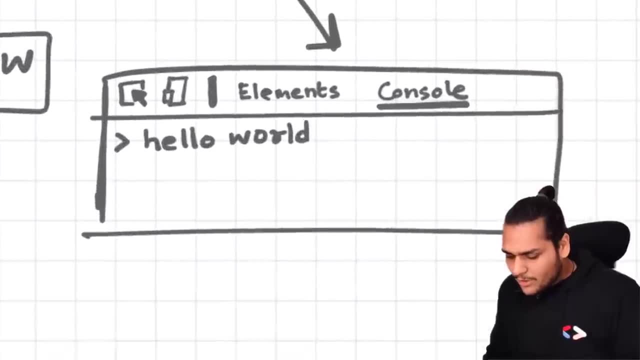 script, it's not javascript, fetch is not javascript, local storage is not javascript. even the console dot log, what you do right, this console dot log, let me just zoom and show it to you. so this console dot log, whatever you do, you see in the browser, that console where you print stuff, it is also not. 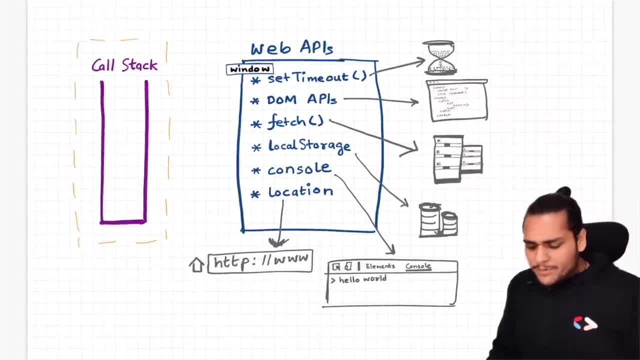 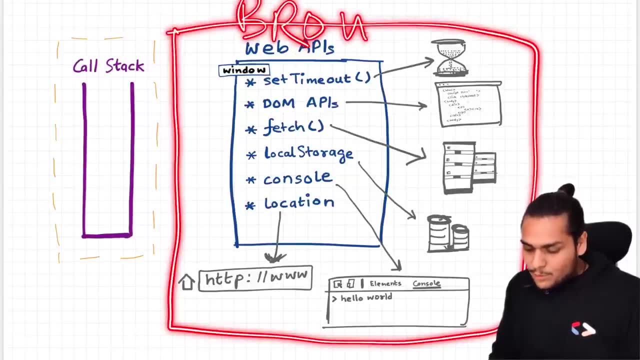 a part of javascript. so these are basically kind of the superpowers which the browsers have it. okay, so these are part of browser. so these are the superpowers which the browsers have it and browser gives us access inside this js call stack, or you can say the javascript engine. 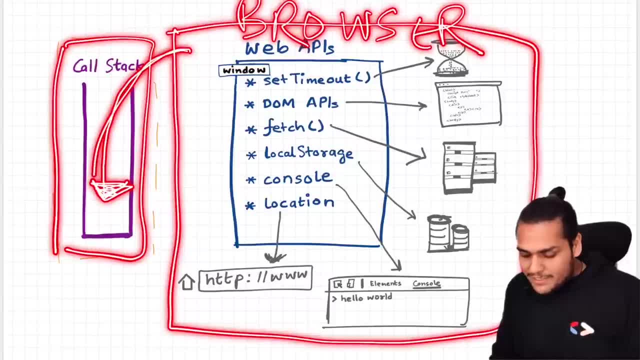 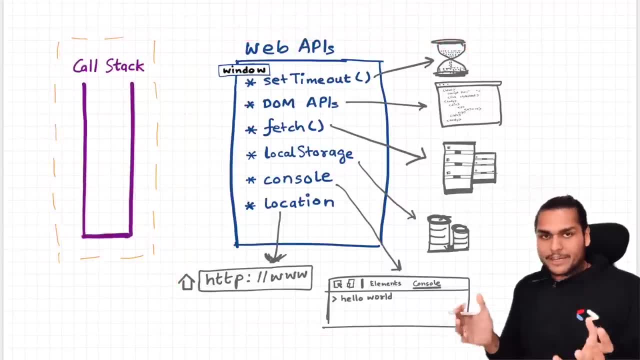 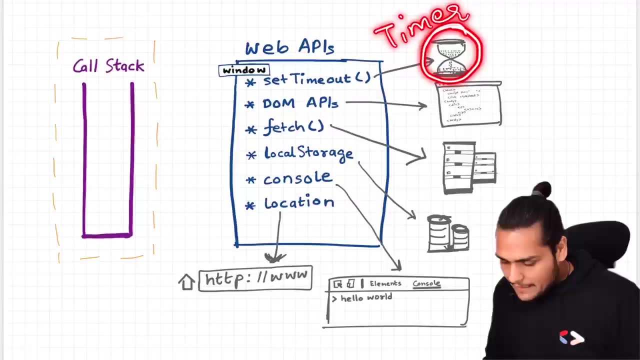 so javascript engine. this browser gives this access to all these superpowers inside javascript engine to use all these superpowers. okay. so suppose if you have to use this timer superpower here we have this timer inside the browser so it gives us access to set timeout. suppose, if we have? 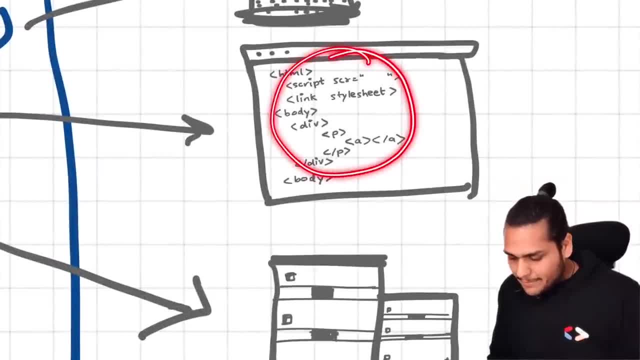 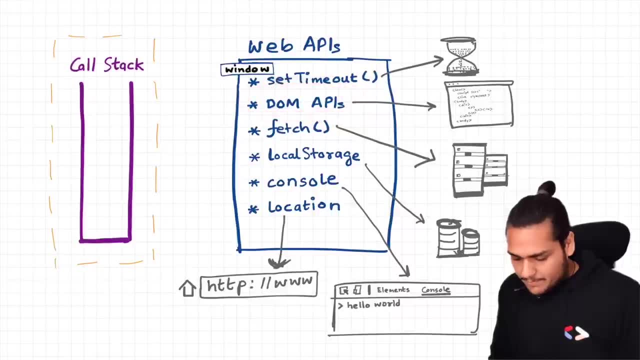 to access this timer. this is dom3 right. this html script rom3. so this browser gives us access to this dom3 by dom apis. so, whatever you do, document dot is the dom apis right. similarly, this fetch gives us access to make connection to the other servers, like the external servers. it's super powerful, right. 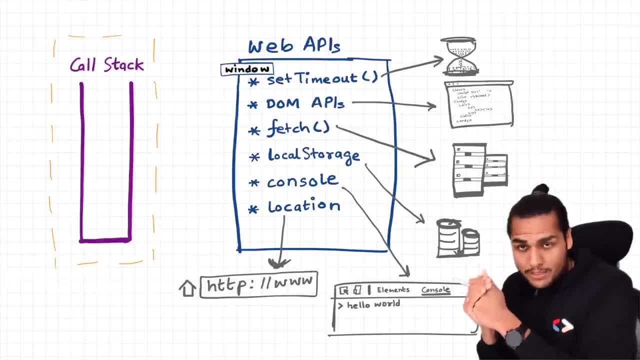 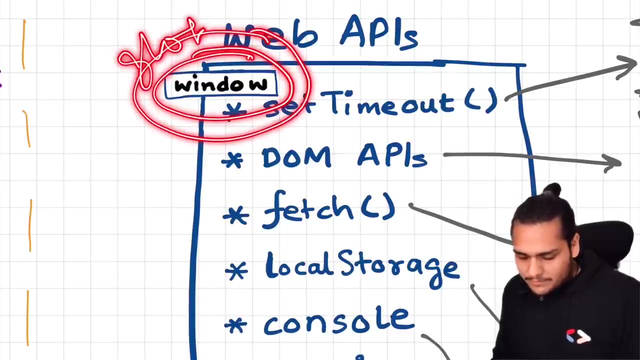 this. all capability is inside, that super power is inside browser. okay, and we get it inside. this call stack: right, because of the global object. now, what is this global object? this global object is this small little window, okay, this keyword, which you see right. this is the global object in case of browsers. browsers give javascript engine. 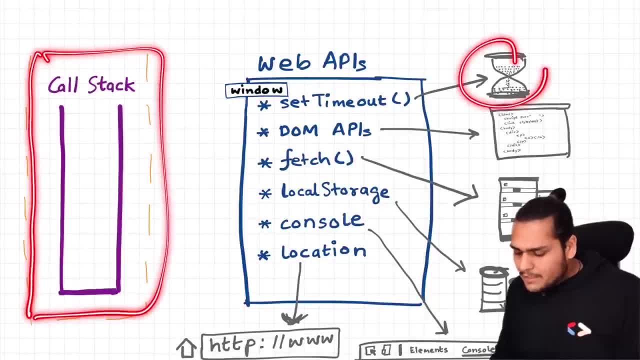 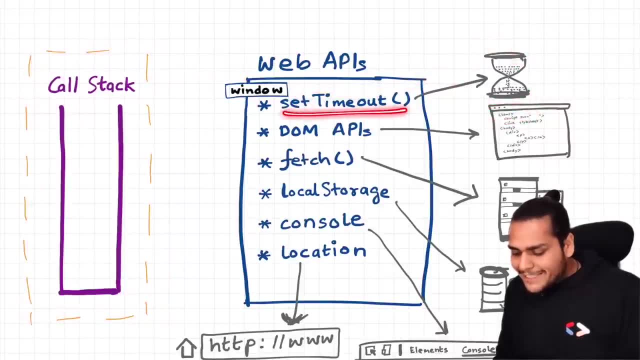 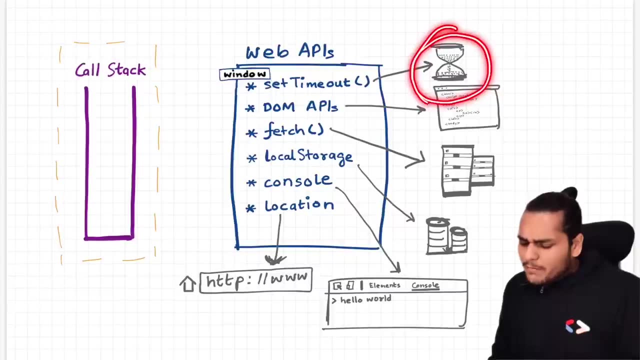 the facility to use all these super powers- okay, this super power of timer, through a keyword known as window. okay, Okay, And all these things which you see over here are the web APIs, Right? So suppose, if you want the superpower of this timer inside your JavaScript code, so you will have to do something known as windowsetTimeout. Okay, If you do a windowsetTimeout inside your JavaScript code, it will give access to this timer. 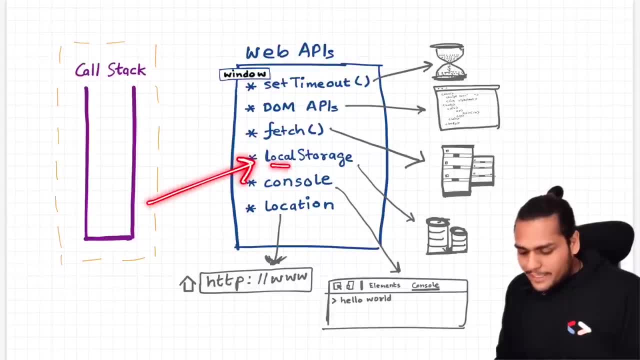 If you do a windowlocalStorage inside your JavaScript code over here, right, it gives you access to this local storage. And similarly, if you do a windowconsolelog, it gives you access to log something inside this console. So that is how you get access to all these superpowers. And there are a lot more. There are a lot of other superpowers. So now, if you ask me that when we write the code, we don't write windowsetTimeout, but we just write setTimeout. 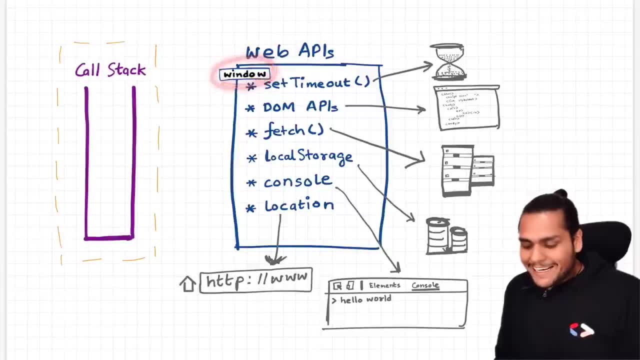 Okay. So because this is the global object and if this setTimeout is present in the global object or at the global scope, you can access it without that keyword window. Right, If you do a windowsetTimeout or you just do a setTimeout, it's one and the same thing. 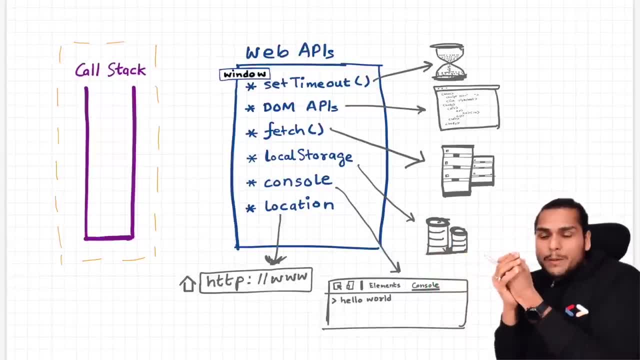 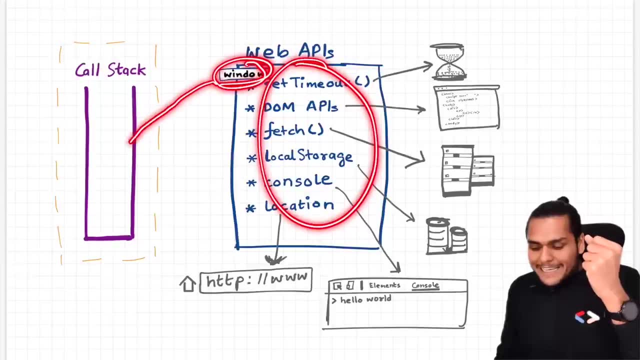 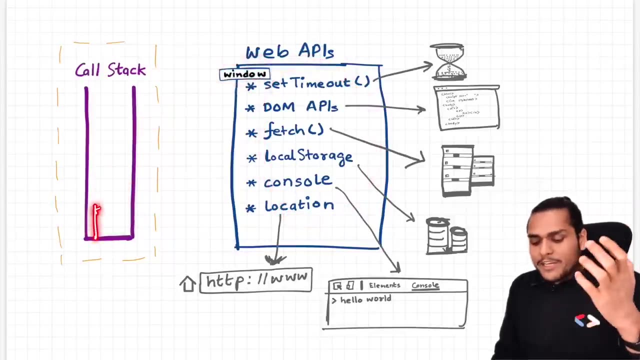 So this browser kind of like, wraps up all the superpower APIs into a global object Right, This global object window. it wraps up all these superpowers and give access of this window to this call setTimeout, stack, or maybe the JavaScript engine, whatever you may call it as, And now in your JavaScript code you can use windowwhatever, or even just setTimeout or fetch or whatever right, to access all these superpowers. 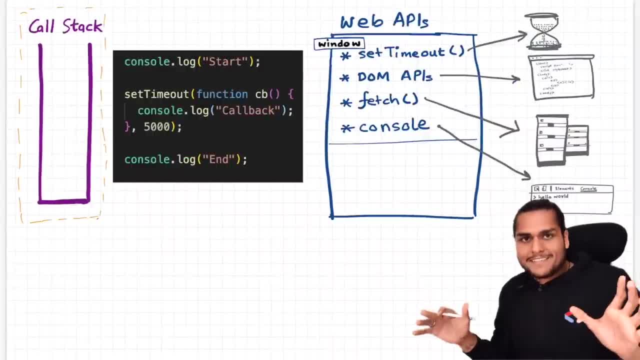 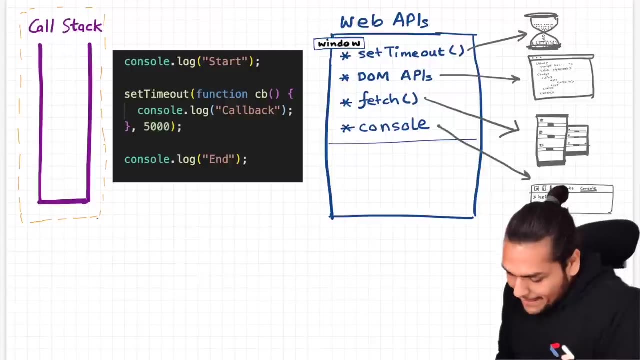 So this was again a lot of theory. Let's move on to the examples. Okay, Now let us try to execute this piece of code and see how it works Using these superpowers. Okay, it will be super fun. Okay, Let's start. So, as I already told you that whenever you try to execute any JavaScript code, a global execution context is created and posted inside the call stack, Let's do that. So we here, we have global execution context. Now this whole code will run line by line. So let's move on to the first line. It's the console log: start. So this, basically, will actually use this API, Right? 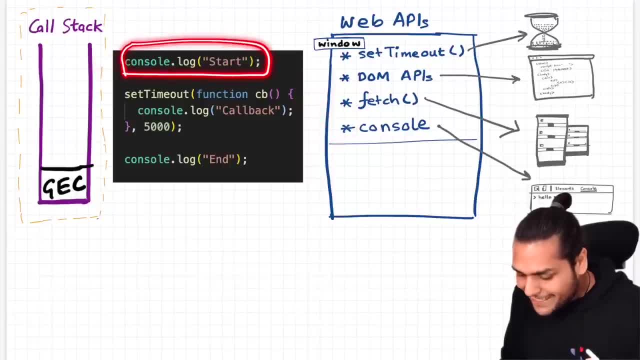 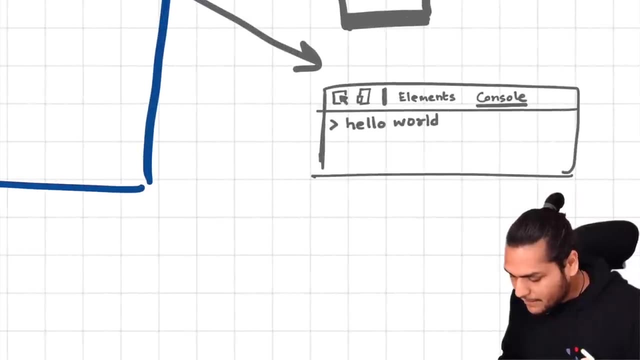 So when you ride console dot log over here in your program, it basically calls this web API And this internally makes a call to actually modify or like log something inside this console, Right? So here we have our console, Right. So this is that developer tools. you right click and do that inspect element and find this console Right. 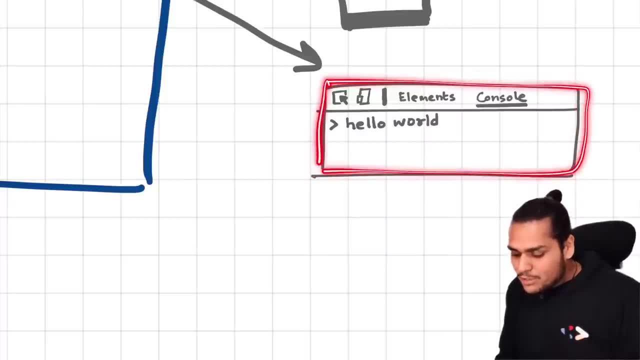 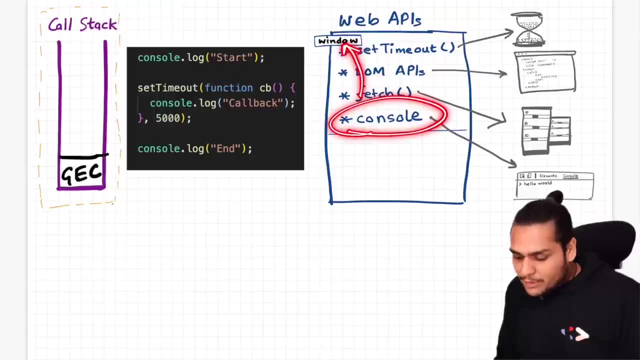 So this console. you can access this console or do a console dot log just because you have this console api. and this api is plugged through window to your code. the javascript code which is executed inside this global execution context got it. so when you execute this piece of code it basically logs into the console let's create. 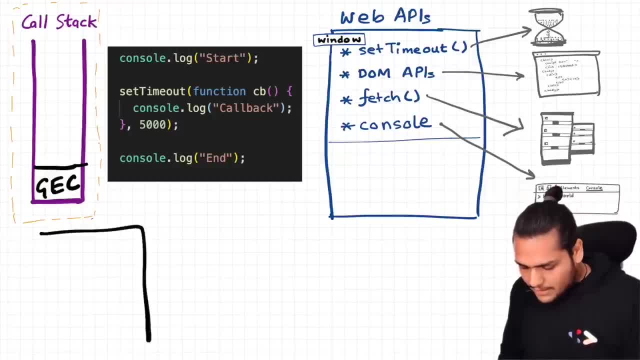 a console, small little console for us. so suppose this is the console, so it will log. start to it. okay, now we move on to the next line. this is the set timeout- what the set timeout will do. the set timeout will basically go and call this web api and this gives us access to this timer. 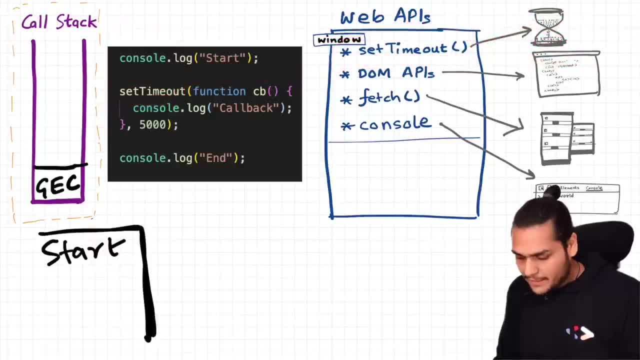 feature of this browser. so this is the superpower by browser, right? so? and it takes a callback function and some delay. so when you pass this callback function to the set timeout, it basically registers a callback. okay, so let me register it. so it registers a callback over here. 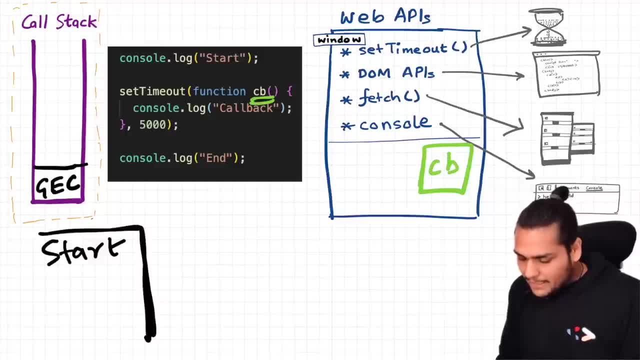 and let's name it cb. so this is the cb callback. it registers this callback over here and, because we pass this delay, so it also starts the timer of 5000 milliseconds inside the timer. okay, in this timer superpower, it starts that 5000 millisecond timer. okay. 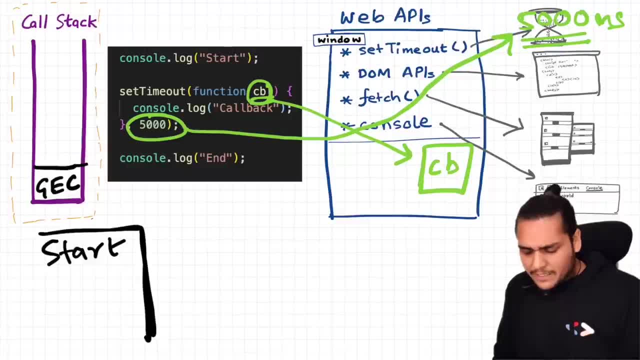 and the javascript code moves to the next line. it does not wait for anything and it moves to the next line and sees this line, consolelog of end, and it logs and it again calls this console and it logs this end into the console. okay, so let's do. 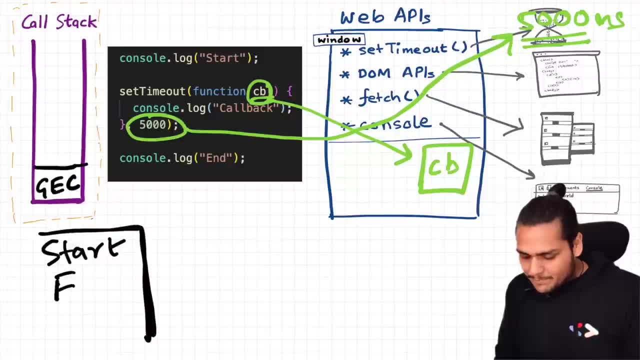 that. so, uh, let's. so this end will be inside this console. got it now? this timer is still running, right. it is just counting, uh, five thousand milliseconds or five seconds and we are done with executing all our code. right, and, once all our code is done, executing the global execution context. 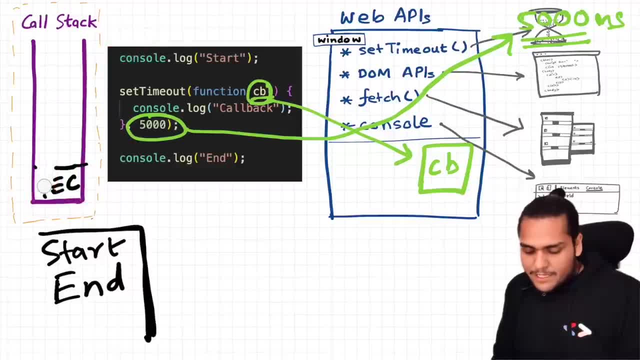 just pops off the stack, right, so this global execution context is gone from the call stack after executing each and every line of this code. and meanwhile all this is happening, this timer is still running. it is doing a countdown of five, four, three, two, one. and as soon as this timer expires, 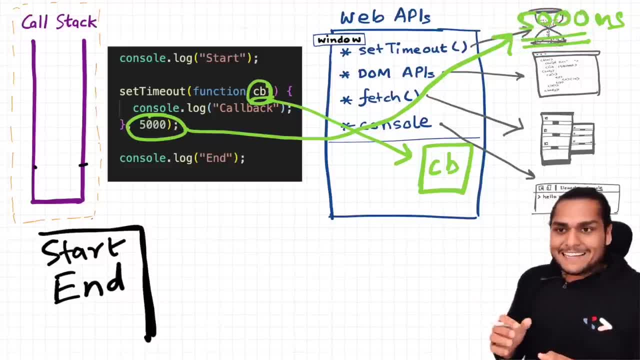 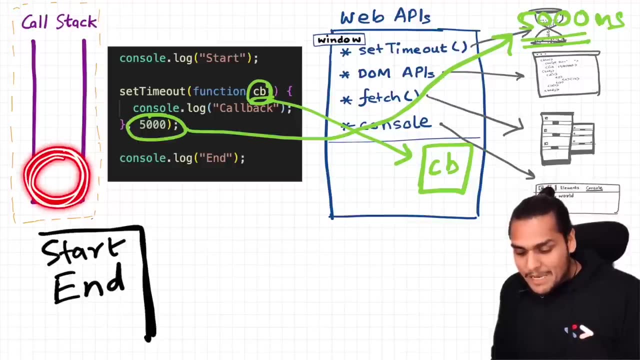 right as soon as the 5,000 milliseconds is passed. okay, this callback function needs to be executed. okay, and because we know that all of the code in JavaScript is executed inside this call stack, we somehow need this callback function inside this call stack, isn't it? so let me just quickly repeat. 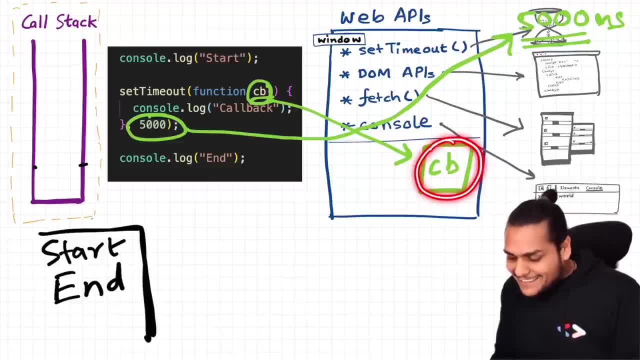 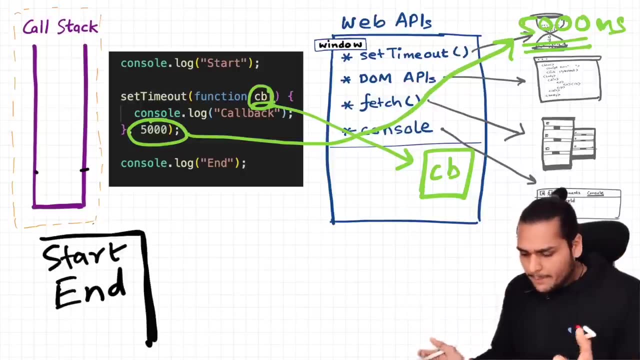 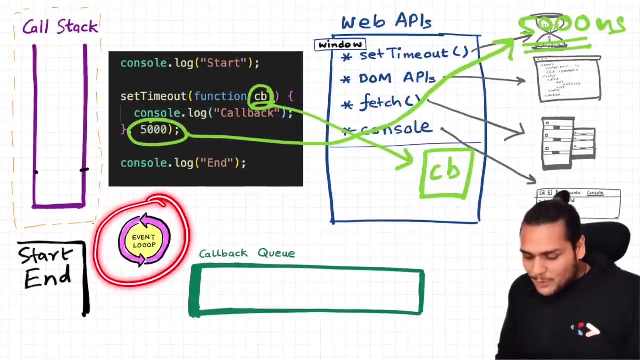 it once again. so if after five seconds we get this callback function somehow inside this call stack, this call stack job is to like, quickly execute whatever comes inside it, isn't it? so now comes into the picture the event loop and the callback queue. okay, let me just draw it quickly. give me two minutes. so here we have our event loop. 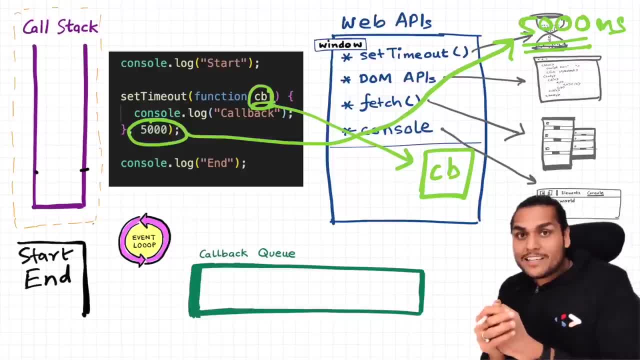 and the callback queue. let us just see that. how does these two things come into picture now? okay, so we already have the callback function inside this call stack and we have the callback function. we already know that this 5,000 millisecond timer was running and this callback was registered as. 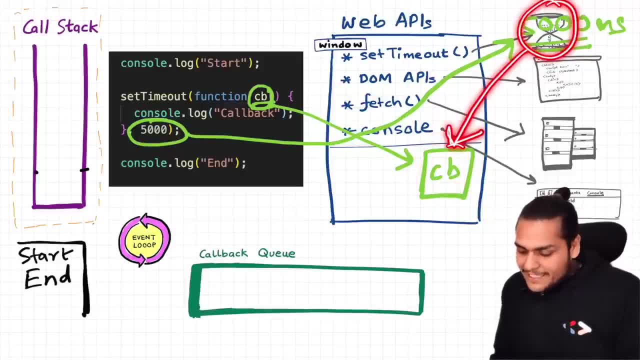 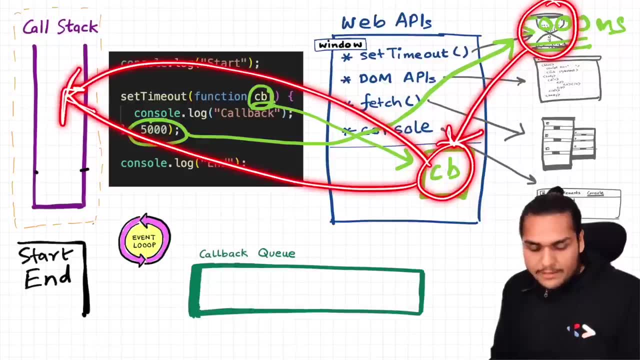 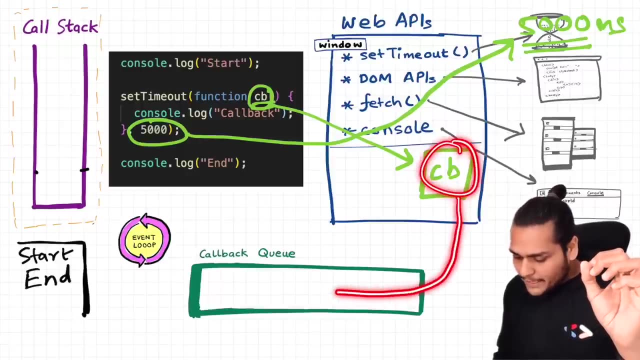 soon as the timer expires. okay, this callback method needs to go inside this call stack, but it cannot directly go into the call stack. then how does it go to the call stack? it will go to the call stack through this callback queue. okay, so when the timer expires, this callback function is. 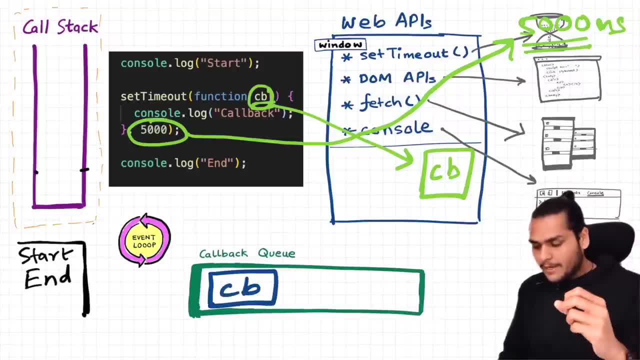 inside this callback queue. okay, so this callback function after the timer expiration moves inside the callback queue and the event loop over here. what you can see. the job of this event loop is to check this callback queue and puts this functions of this callback queue into the call. 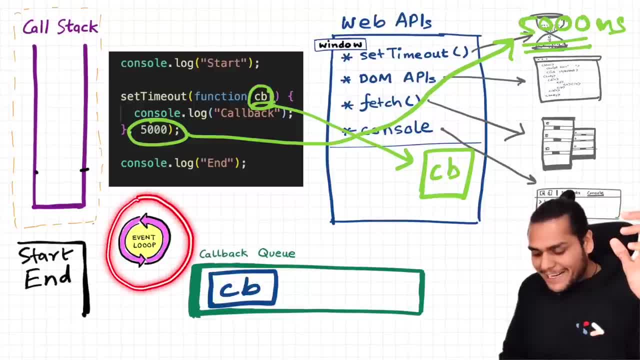 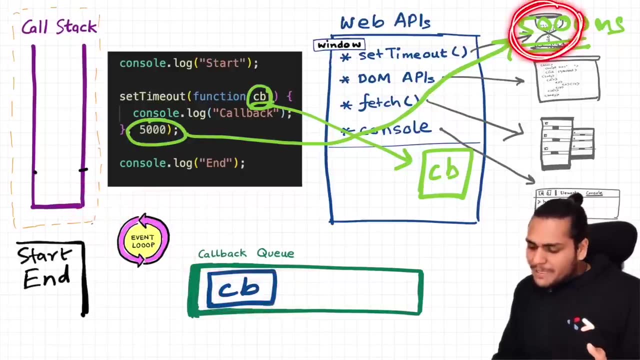 stack. so the event loop over here acts like a gatekeeper and it checks whether we have something in this callback queue and if we have something, just like our callback method, it just pushes that inside the call stack. okay, so as soon as this 5,000 milliseconds timer expire, this callback 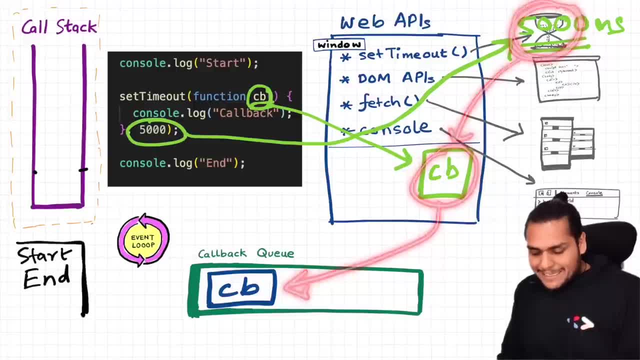 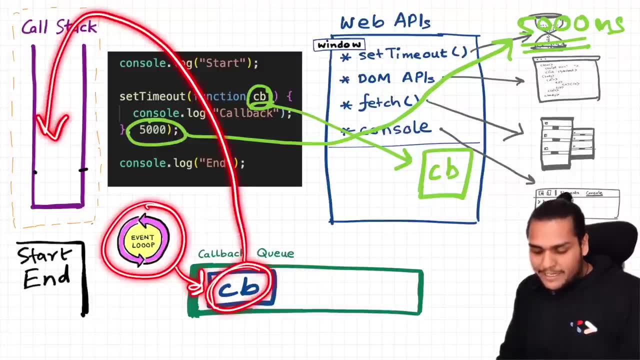 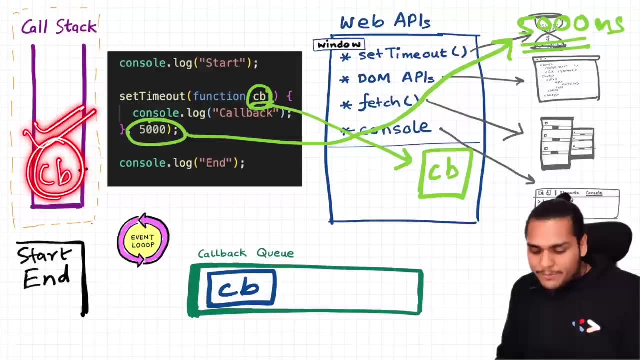 function over here is pushed inside the callback queue and event loop checks whether there is something inside callback queue. it finds this callback method and it pushes inside the call stack and it and that call stack quickly executes this callback function. okay, it executes function how. it creates an execution context, pushes that execution context of. 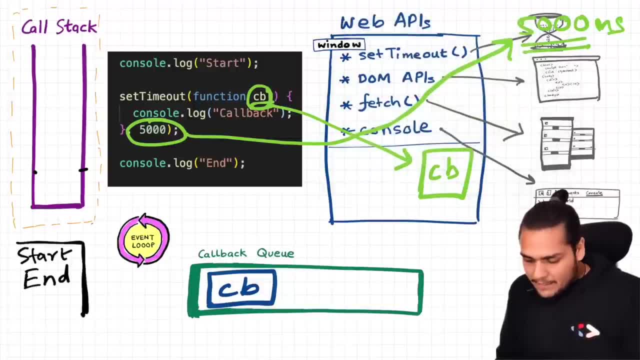 that CB inside it. let's do it quickly, okay. so it pushes that callback function execution context and it runs this callback function line by line over here. it just has one line. it sees that console log of callback. when it sees the console log it goes to the console and this console web API actually logs it. 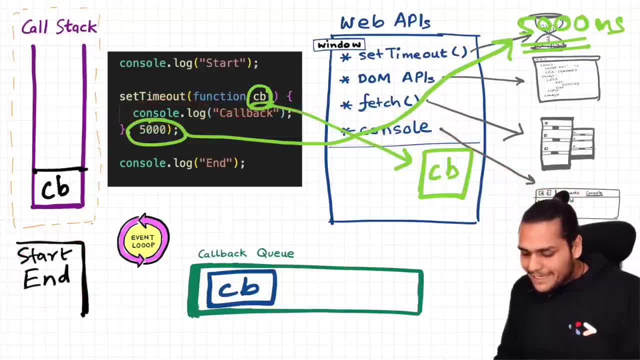 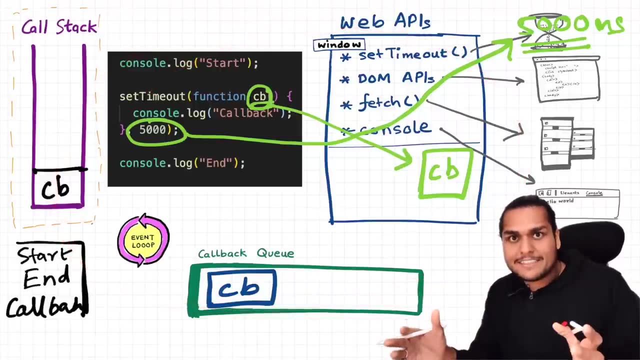 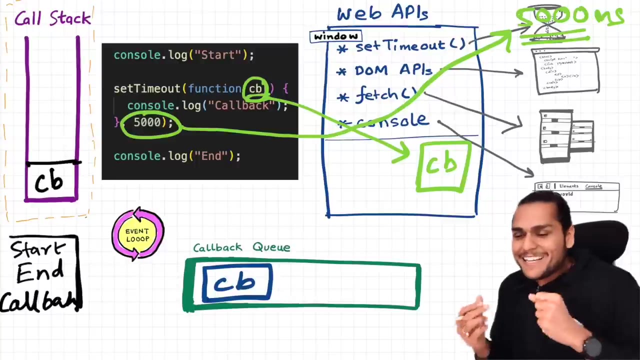 into the console and our console is over here, so let's log callback inside it. so this callback string will be logged inside console and that's how, my friend, this whole thing works. I know this will be very confusing to a lot of people. that is why I have come up with many more examples. so let us dive deep. 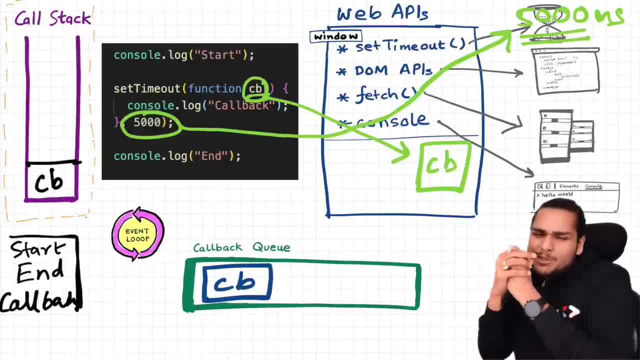 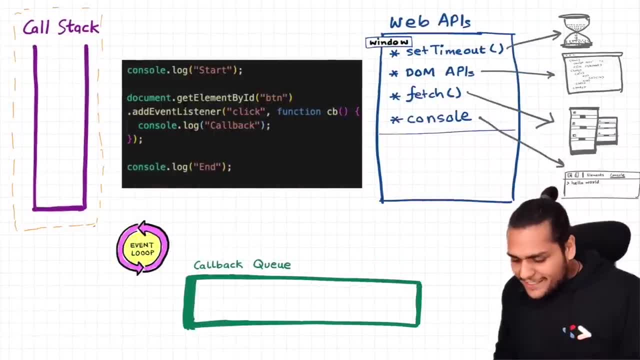 into those examples and this concept will like become stronger and stronger in the future In your head. okay, let's just do that quickly, it will be super fun. so if we move on to our next example, so now we have this piece of code. okay, so now clearly see this piece of code. so over here, what we do, we do a console. 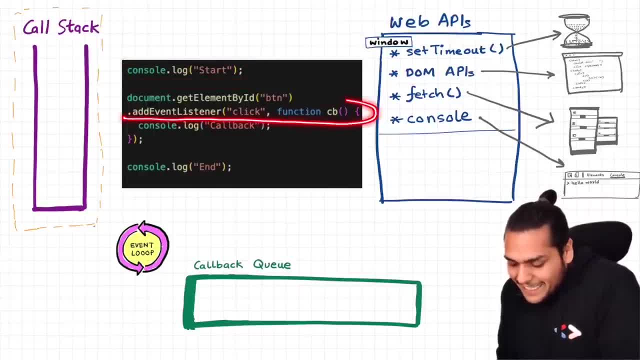 log and we have a event listener inside our browser this time. okay, this is basically document dot get element by ID BTN and we have put a click event handler inside a button. so suppose if we have a button inside a button and we have a click in our button, we have a click in. 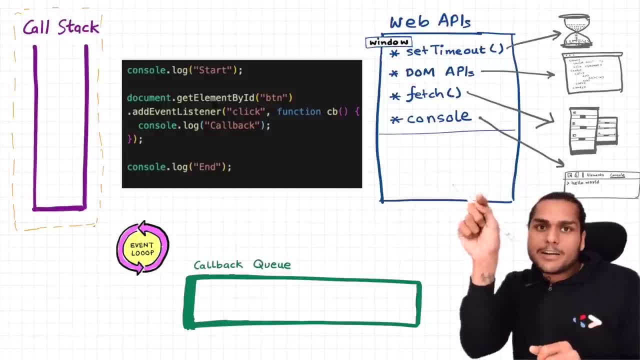 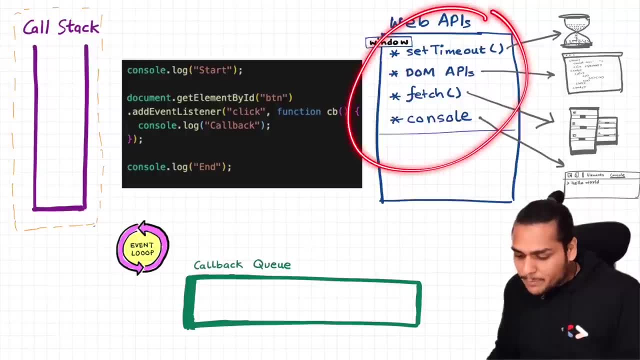 inside our web browser and if we want to do something on the button click. let us see how that works behind the scenes. okay, and how does all these web api's come into picture? in that case of event handler, when we click on a button, what happens? okay, so again, whenever you run any javascript code, what happens? yes, the 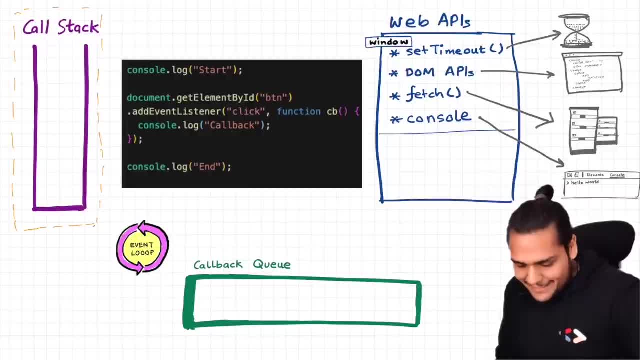 global execution context is created and pushed inside the call stack, isn't it? now you might stuff like memorize it, right? so this global execution context is created and this is put inside the call stack, right, and the code is executed line by line. it moves to the first line. it sees the console log start. 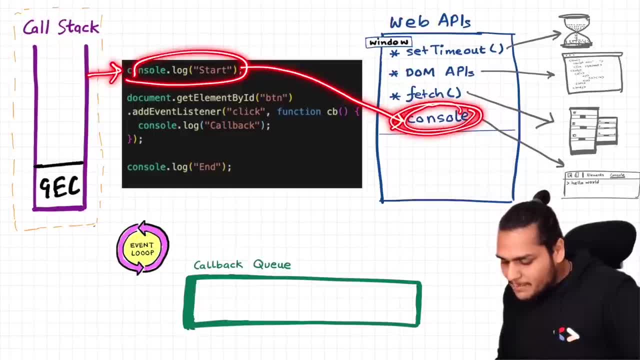 and it goes to the console. it sees it calls this method web api method, and it logs something to the console over here. so let us make our console first of all, so we have this console with us. okay, so this is our console and we log start. okay, so this is our console and we log start. 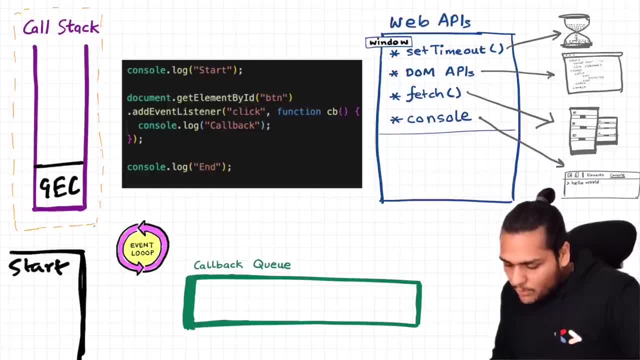 okay, so this is our console and we log. start over here. got it now. it now the code moves to the next line. now this is document dot. get element by ID: BTN dot. add event listener. now, what is this add event listener? this add event listener is another superpower which is given by 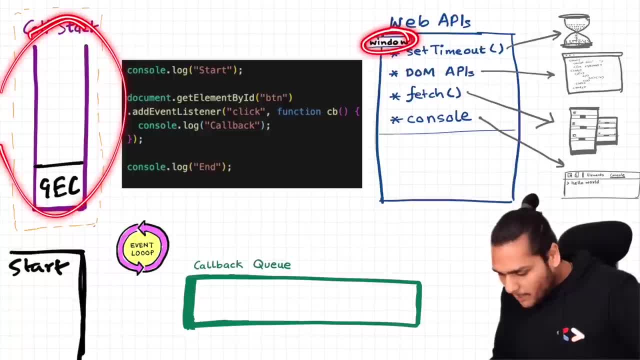 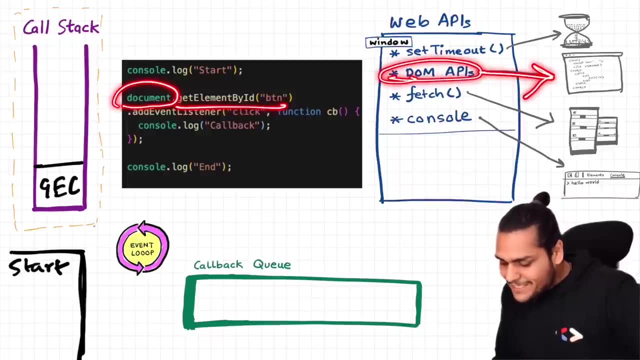 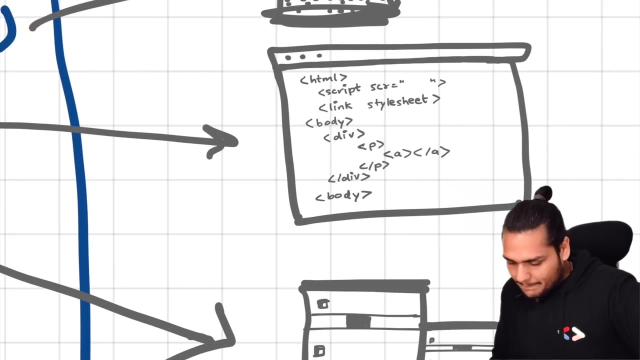 the browser to the JavaScript engine through the window object in form of a web API, which is the Dom API, right? so whenever you do something like document dot, it basically is calling this Dom API, which basically, in turns, fetches something from the Dom. okay, Dom is the document object model. it is like the HTML source code: see see. so 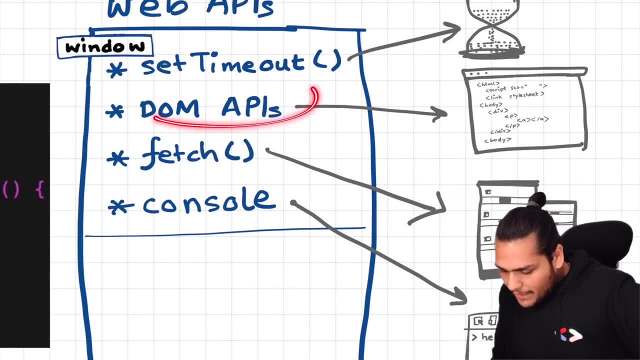 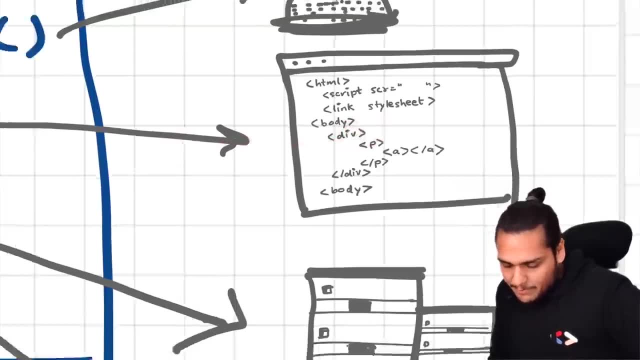 whenever you access this Dom API. okay, so this Dom API, it basically access this HTML code and tries to find out a button with some ID and it returns it something like that. okay, and if you put in this dot add event listener, so it also registers a call. 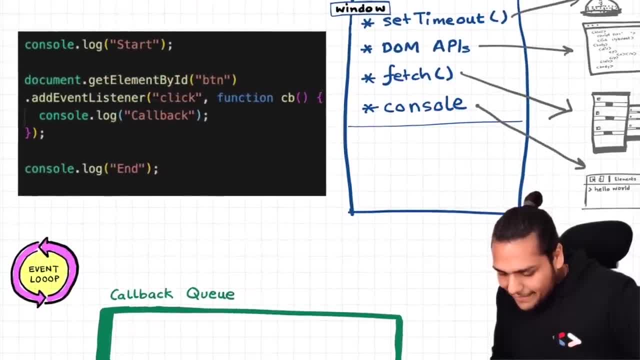 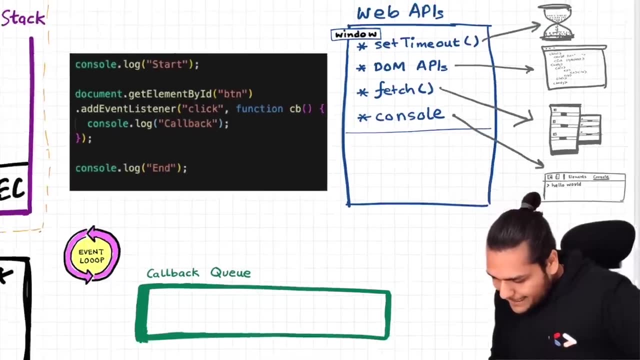 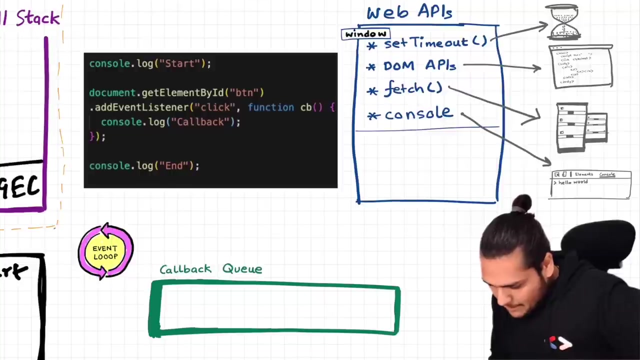 back right? this event listener, this add event listener, registers a call back on an event. that event is click. okay, let me show you how it does. what it will do is it basically over here. inside these web API is environment. so inside this web API is environments. a callback will be registered. so that callback is the CB. 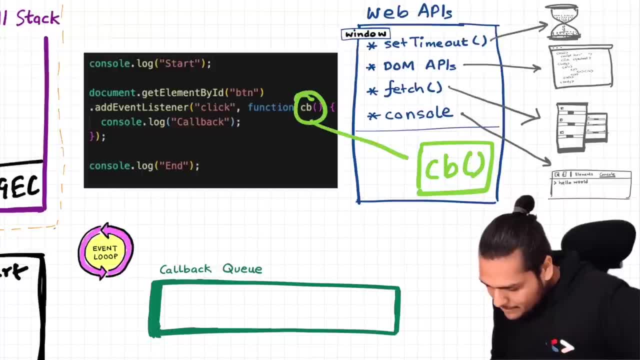 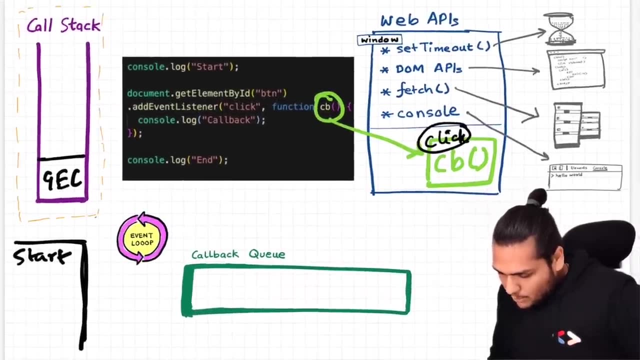 right. this callback is this method right? this callback is registered over here and an event is attached to it. that event is the click event. okay, so this is known as registering a callback. okay, so in the web API is environment. whenever you see this line, add event listener it. 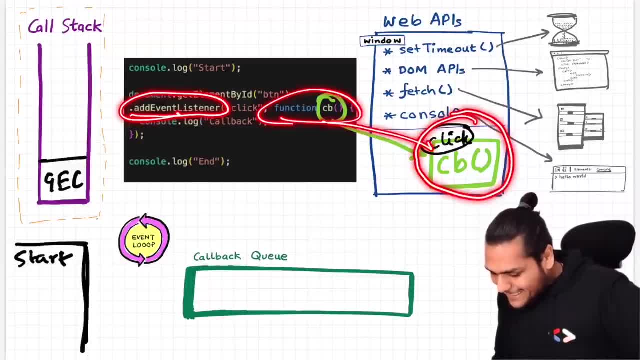 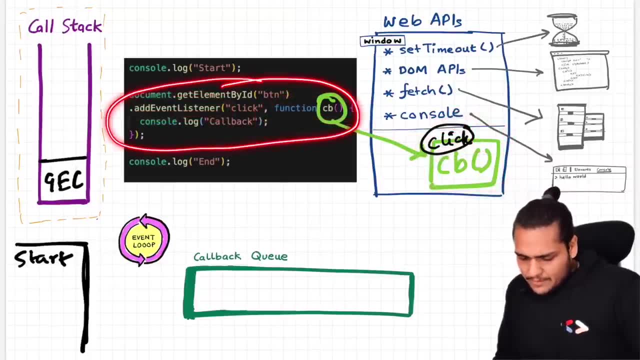 basically registers this callback method right and attaches an event to it, that is the click event and that's all in this line, attaches the event handler quickly and then it moves on. JavaScript waits for none, right, it start executing the next line. so the next line is console log end. 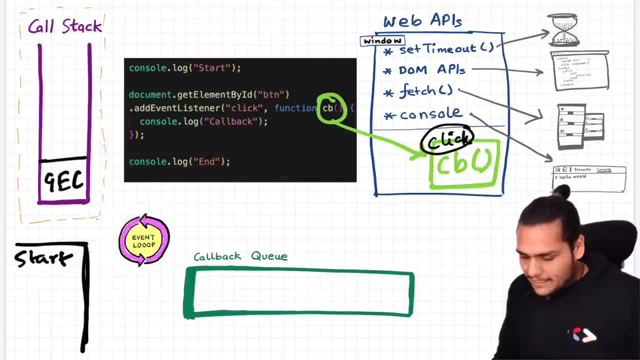 and it basically logs: end over here, right, so let us just do that, so we have end inside our console now. then we have nothing more to execute over here. so this global execution context also like pops off the start. it's gone, right, let me just remove it. so now this global execution context is: 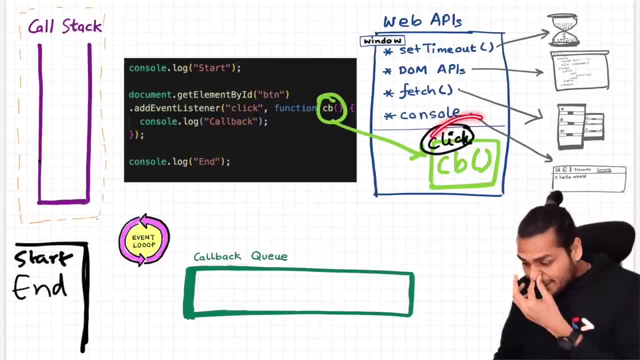 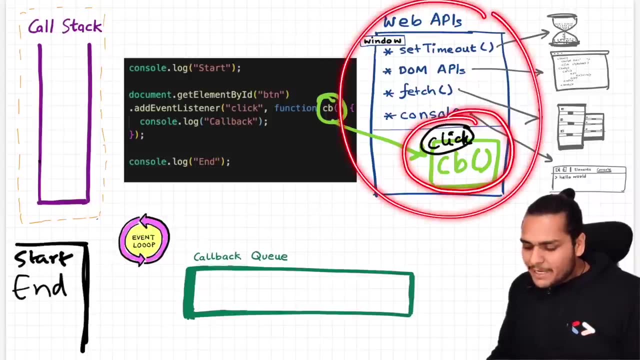 gone, but this event handler will stay over here in the web API is environment until then, unless we explicitly remove that event listener or, we like, close the browser. so this registered callback method inside the web API is environment just sits over there and in the hope of that, some user will someday click on the. 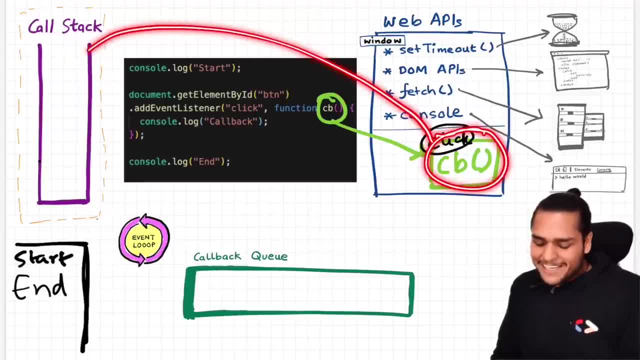 button and this callback method will see the light of the day and move inside the call stack to execute. it just waits over there, right when the user clicks on the button. this callback method is then pushed inside the callback queue. and this. let's do that. ok, this callback method goes over here and sits inside the callback queue and it. 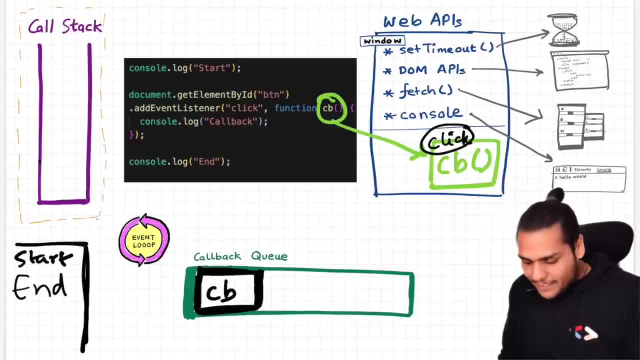 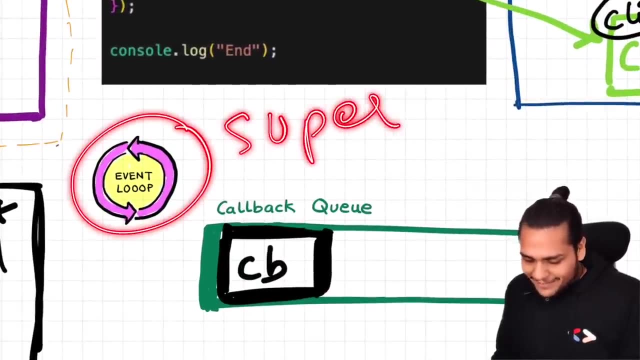 waits over here for its turn to get executed. ok, so now let me explain you a little bit more about this sweet little event loop. right? so this whole video was dedicated to this superhero event loop, right? this is our superhero right of the evening. let's see what it does. 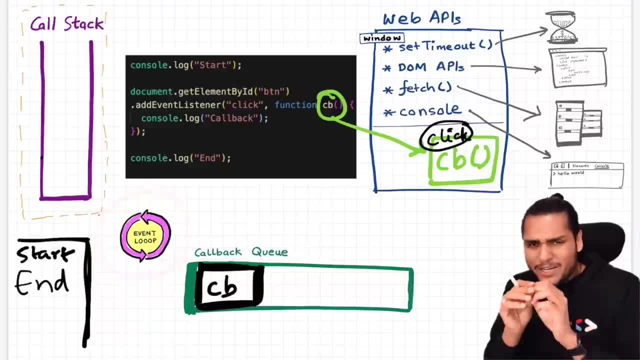 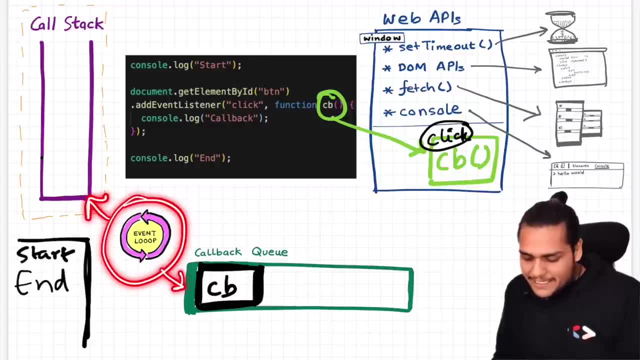 so, basically, you know, event loop has just one job. okay, its only job is to like, continuously monitor the call stack as well as the callback queue. so if this call stack is empty and this event loop sees that there is also a function waiting to be executed inside this callback queue, 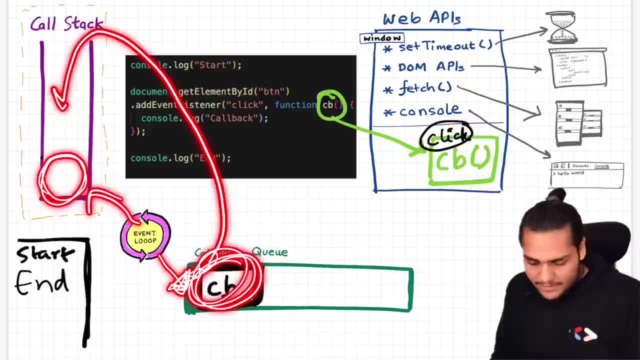 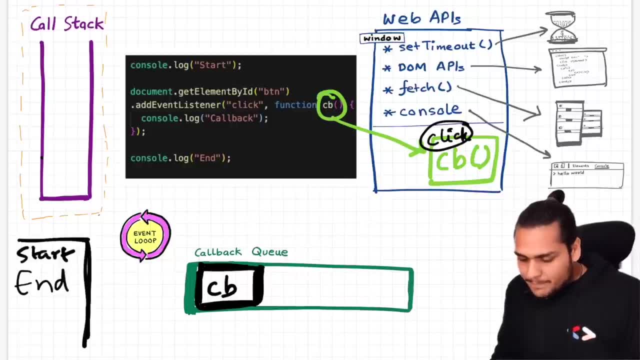 it just takes this function and just push it inside the call stack and the callback method is like quickly executed, then right, so let's do that. so this callback method now goes inside this call stack and it is like quickly executed, so it runs the code line by line, this code line by line. 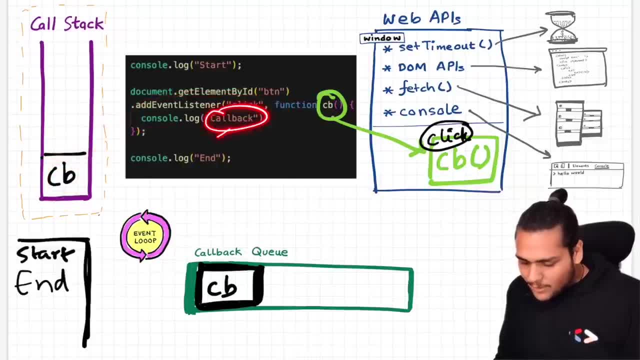 it just sees that console log of callback. it prints this callback inside this console. let's do that quickly. callback right and it's gone. right and it's gone from the callback to the callback. and it's gone from the callback to the from the call stack. okay and sorry, i missed it. when the event loop picks it up from the callback, 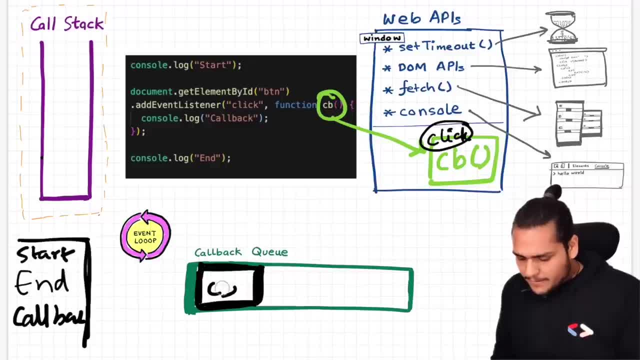 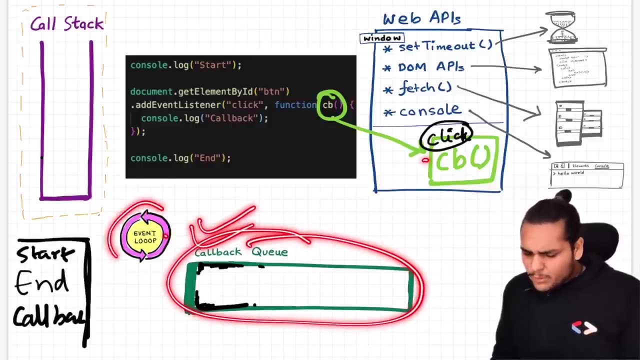 queue. it just vanishes from here. also, let me just remove it. okay, so that's how this callback method is executed when the user clicks on it. now an important question comes to our mind, that why do we need this callback queue? right, we can just directly event loop, could have directly like 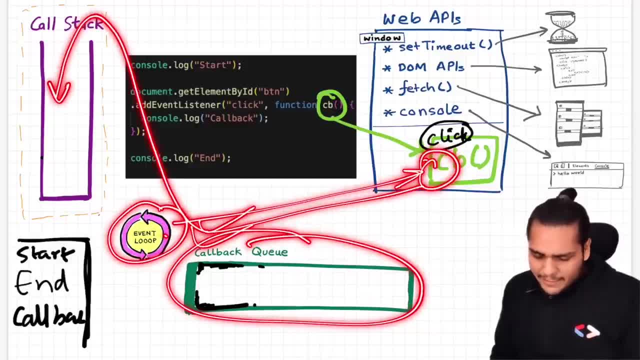 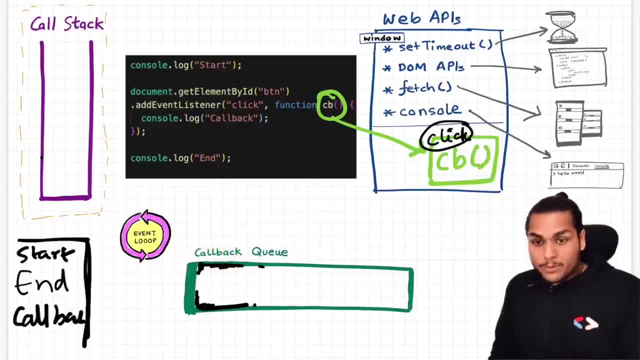 picked up this callback and just put it inside the call stack right whenever the call stack is empty. but no, we need a callback queue. why do we need a callback queue? so suppose that user clicks on the button like seven, eight time, continuously like, click, click, click, click, click, right in that case, 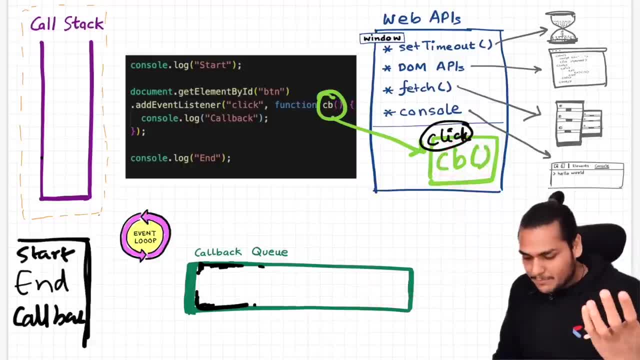 this callback function will be pushed inside this callback queue five, six times. there will be five sick callback function waiting to be executed inside this callback queue. let me show you how will it look. so then we will have this callback function over here, suppose the user clicks it. 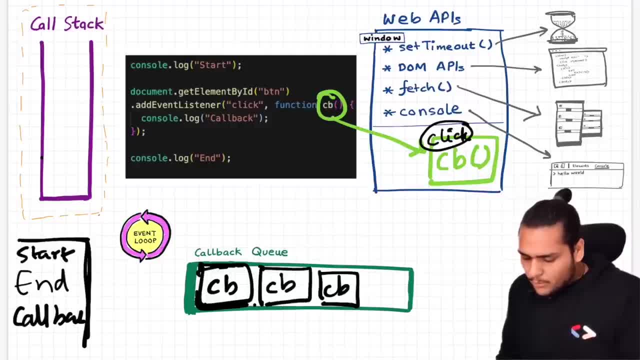 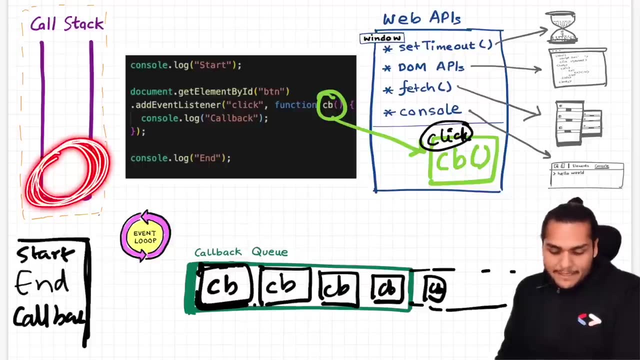 continuously right, Right. So we will have a queue Right. We will have all these callback functions waiting to be executed And our event loop friend Right. This friend will continuously check whether the call stack is empty or not And if that call stack is empty and there is some function lined up to be executed in the call callback queue. 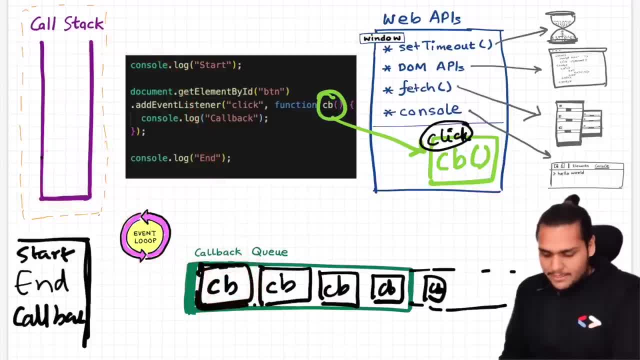 So it takes that function and pushes inside call stack and it executes And slowly, slowly, this pops off the callback queue and slowly, slowly, it executes all of these callback functions one by one. So generally in a real life application we often see that there are a lot of event listeners and a lot of other things happening inside the browser. 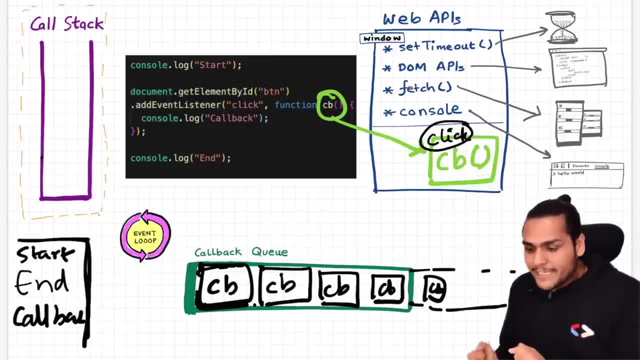 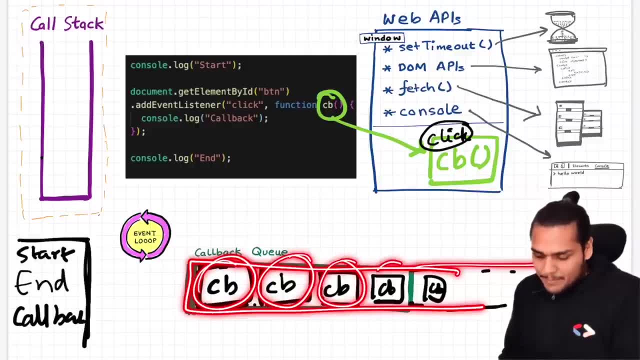 Right, A lot of timers, a lot of event listeners. So that is why we need to queue all of these callback functions together, so that they can get a chance one after the other, Because JavaScript just has this one call stack Right And everything in JavaScript is executed here only. 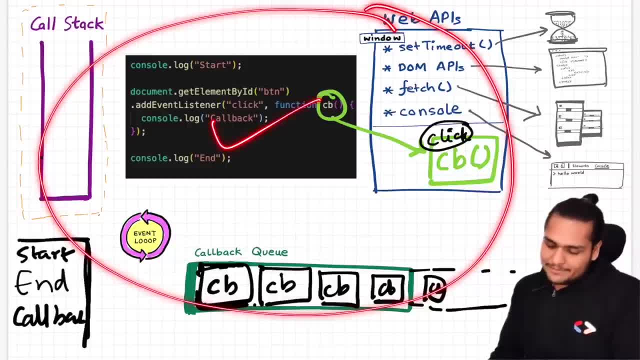 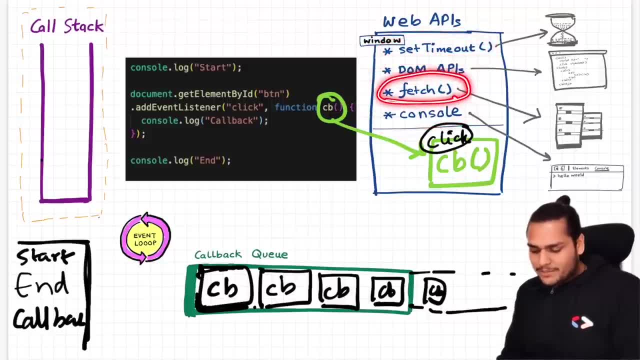 Isn't it? So that's how this whole thing works. So we have already seen that, how set timeout works, how DOM API works, how console works, But we haven't seen how fetch works. So fetch is an interesting case. So fetch does not work the same way as this event, listeners or the set timeout. 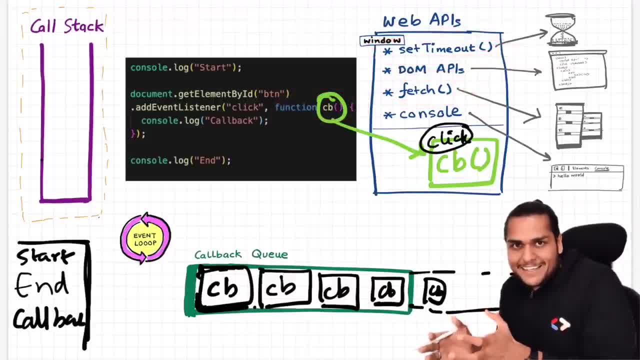 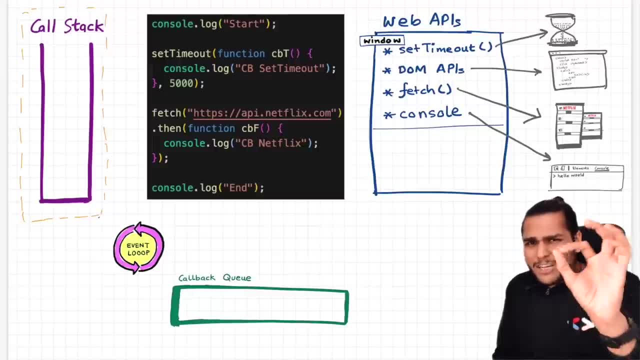 It works a little different. Let us also see that. Let's take one more example to strengthen Our concepts more deeper. Okay, let's go dive deep more into it. I know this might be too much in a single video, but give me just five more minutes. 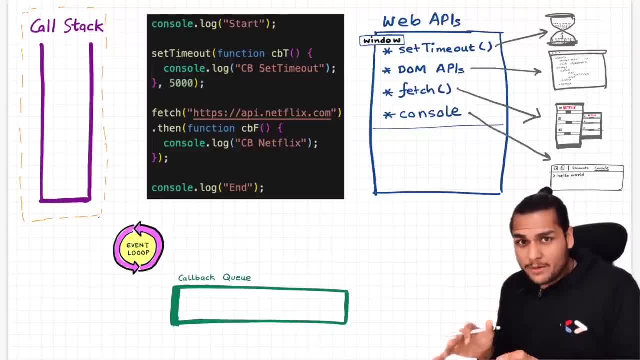 This example is very important and it is very unique. Okay, just bear with me for five more minutes. Okay, so let's see now. So this time in our code we have set timeout as well as our fetch function. Okay Now, if people who don't know what fetch is, fetch basically, goes and request an API, 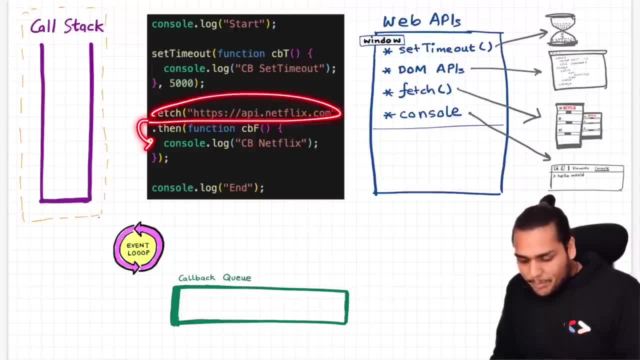 I call Okay. so this fetch function returns a promise and we have to pass a callback function which will be executed once this promise is resolved. Okay, so I haven't covered promise yet. But when we, when I say promises resolved, that means that when we get this data, 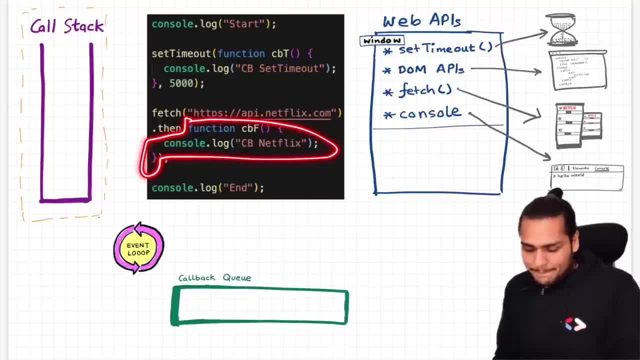 then we actually just execute this callback function. Let's see all this in action. Okay, So, just like the same old story, a global execution context is created, pushed inside the callback stack. The code is executed line by line. We do a console log of start. 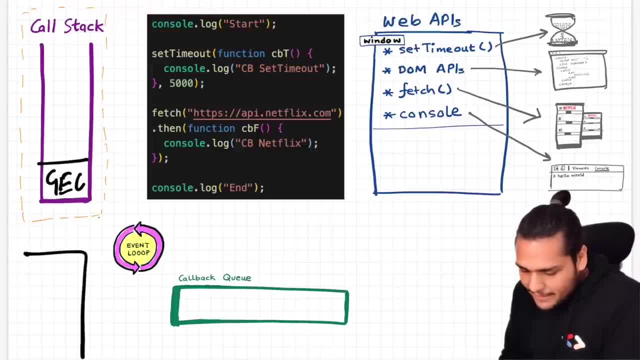 It prints it into the console. Let's just create a console quickly and just print the start over here. Okay, Now it moves to the next line and we already know what will happen. The set timeout will basically register this callback function right where in the web APIs. 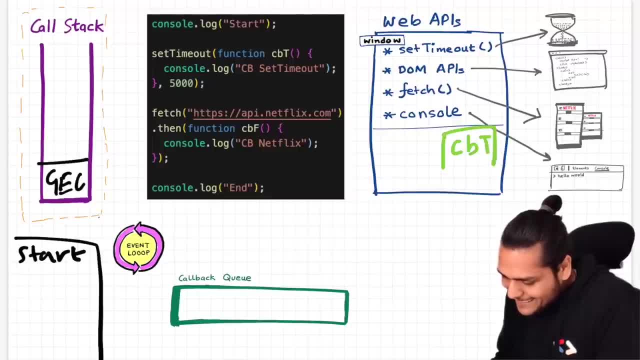 So we have the CBT inside our this function right In Registered inside the web. API is environment and we also have the timer of 5000 started right. this 5000 millisecond timer starts and the JavaScript engine then moves to the next line. 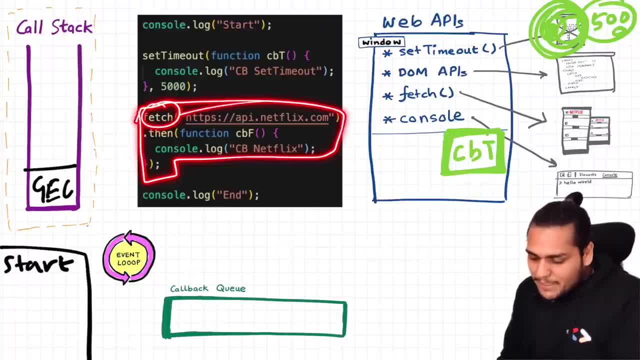 So now we have this fetch function. This fetch is again a web API which is used to make network calls. Okay, so it basically also registers this callback function into the web APIs environment. Let's register this CBF, This callback function, CBF, inside our web APIs environment. 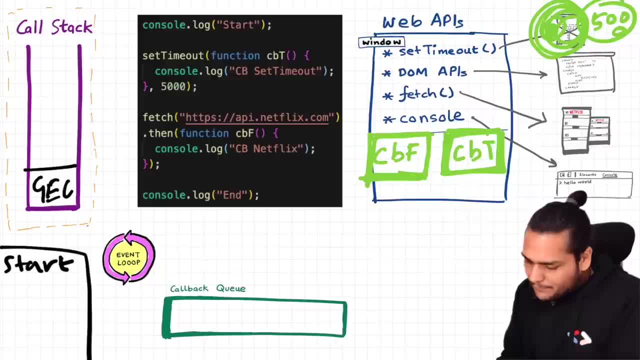 Now we have these two functions sitting over here: CBF and CBT. The CBT function is waiting for this timer to expire so that it can see the light of the day through the callback queue, and CBS function is waiting for data to be returned from this. 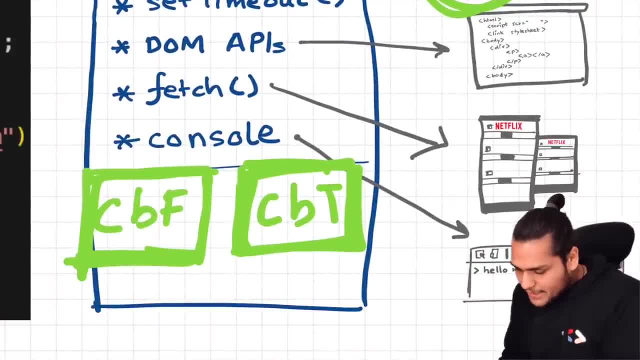 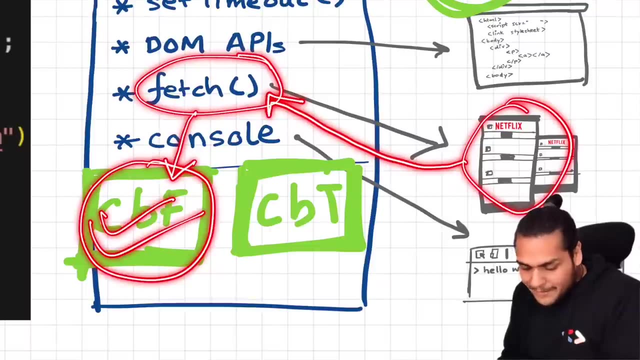 Netflix servers. So let's zoom in. So this fetch function will basically make a network call to this Netflix servers and this Netflix servers will return the data back to fetch And once we get the data over here, this callback function will now be ready to be executed. 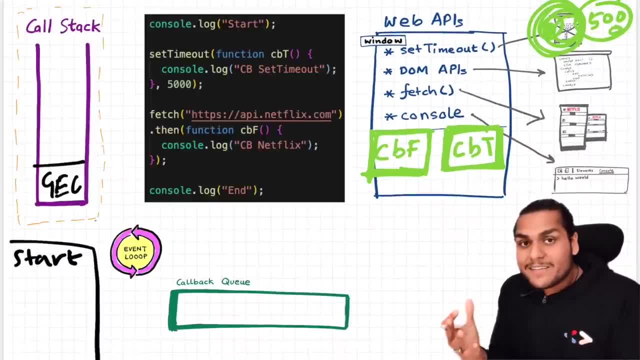 Got it. So suppose this Netflix servers are like super fast and it returns the data within like 550 milliseconds? Okay, let's say, after 50 milliseconds we got the data from the Netflix servers over here right Now. this callback function is ready. 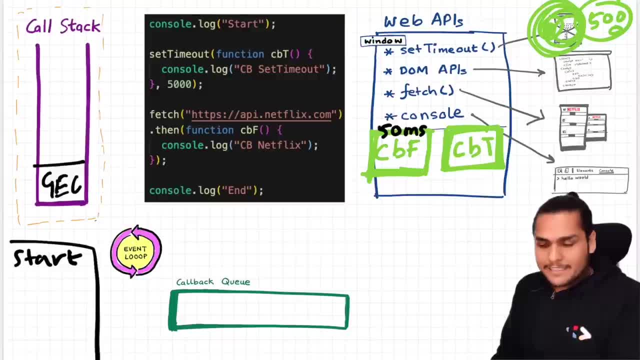 To be executed, Isn't it? What do you think will happen? This callback function will go to the callback queue. That is what you expect, but no, that won't happen. Now comes the most confusing part, which a lot of developers don't understand. 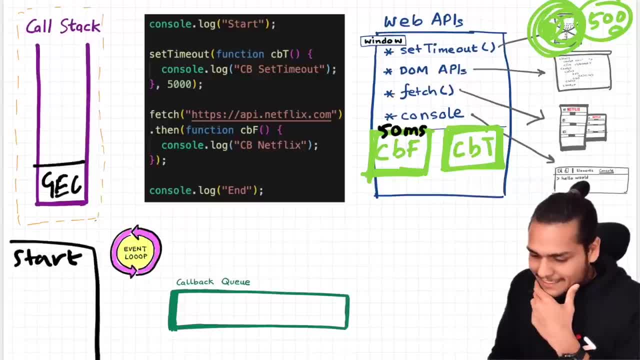 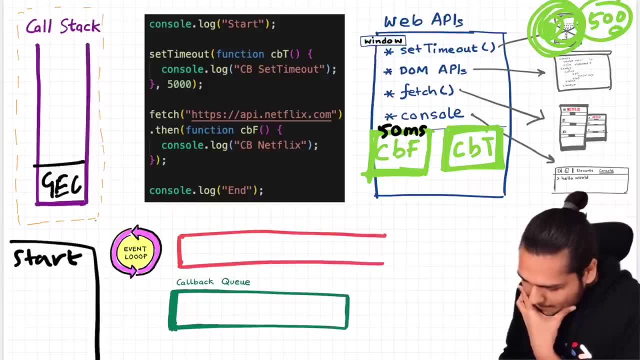 That is the micro task queue. Just like this callback queue, We also have something known as a micro task queue. Okay, Here we have this micro task queue. This queue is basically exactly similar to this callback queue, but it has higher priority. 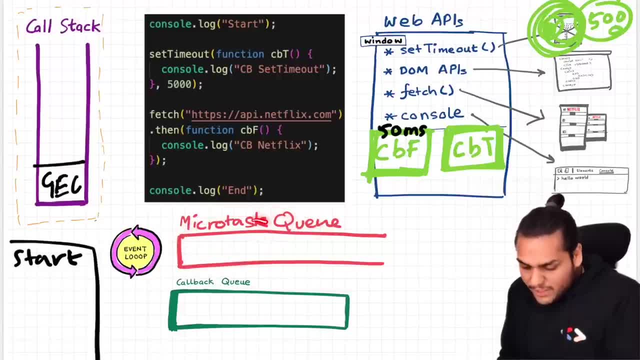 So this queue has higher priority. Whatever functions come inside this queue will be executed first, and functions inside the callback queue are executed later. Okay, Now what comes inside micro task queue? Yes, you guessed it right. This function CBF over here, which was a callback function in case of promises, right? 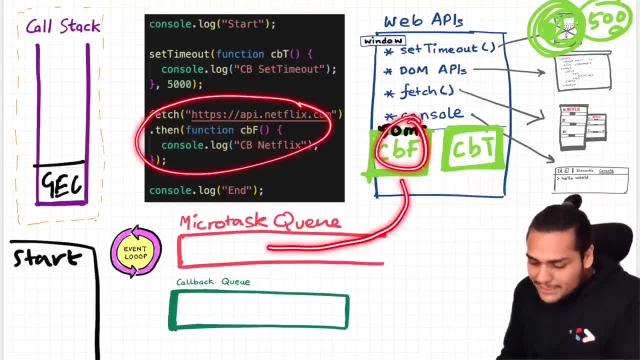 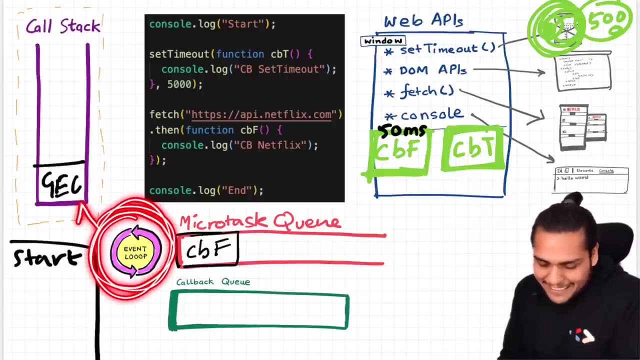 In case of this, network calls will go to this micro task queue. Okay, so this callback function, CBF, will go to this micro task queue And again, the job of the The event loop is to keep on checking whether the call stack is empty or not. 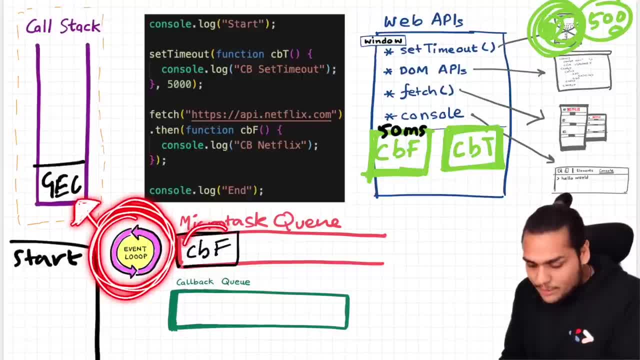 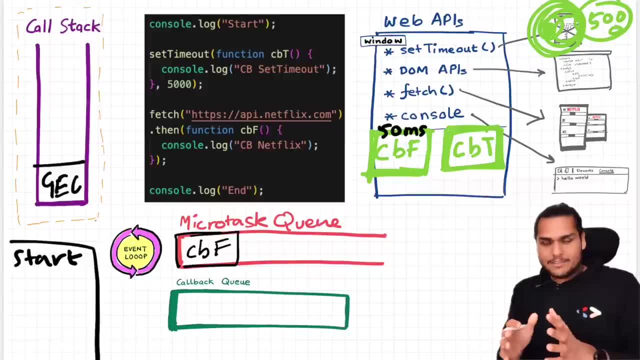 And once the call stack is empty, then it gives the chance to all these functions over here in the queue to see the light of the day inside the call stack. That's how it works. Okay, So right now we are not done yet executing this code, right? 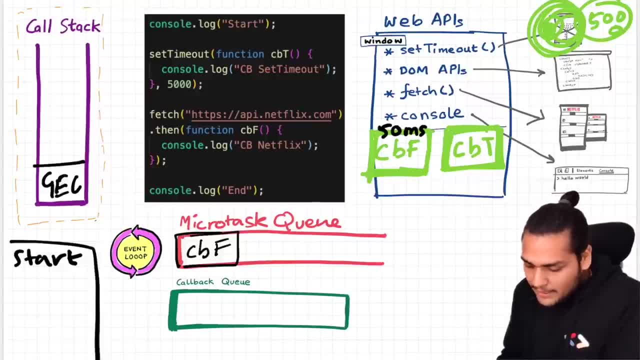 So we were still executing this code. This line was still left, but we already got the response from the Netflix servers. They were very fast, right Within 50 milliseconds. We got the response, but we are still executing this code. Suppose there are thousands of line in the code. 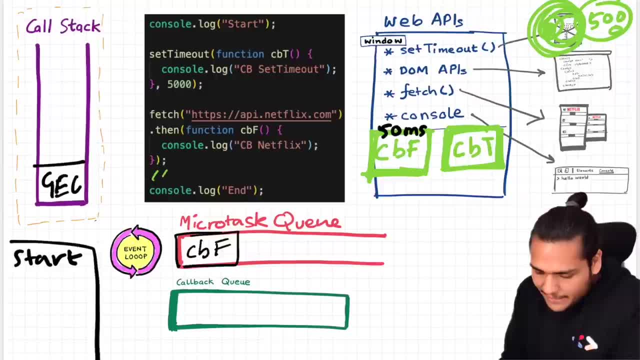 Okay, let's make it to understand more clearly. Suppose there are a lot of lines, Suppose we have millions of line over here, millions of line of code- Okay, and it takes some time to execute this, right, But we already have this callback function waiting over here to be executed. 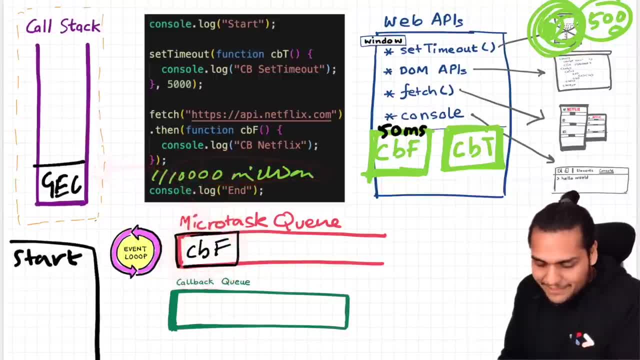 But we are running these millions of lines of code in our main thread, right, Let's see when it gets the chance. Meanwhile, we are running these million line of code. The timer also expires, right? The browser isn't doing just one thing. 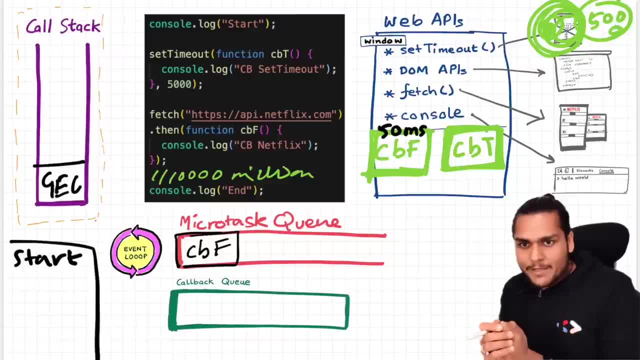 It is just the JavaScript engine which is doing one thing at a time, But browser is doing a lot of things behind the scenes, right? This timer is also ticking up, So once this 5000 millisecond expires, this callback function- callback T- basically wants to be executed. 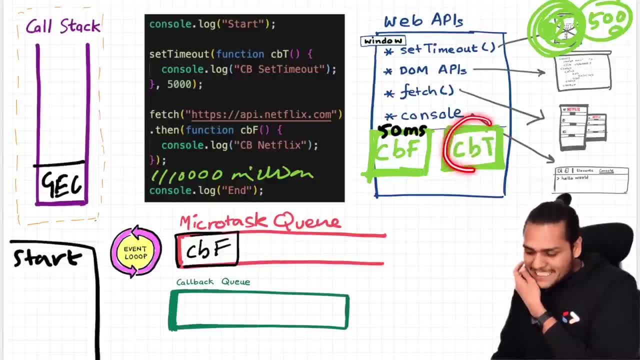 Now This is ready to be executed. How will this be executed? The same process: it will go inside the callback queue. Let's move it inside the callback queue. the CBT, the callback from the timer. It goes inside the callback queue. Now, this million line of code is still executing. five seconds have passed. 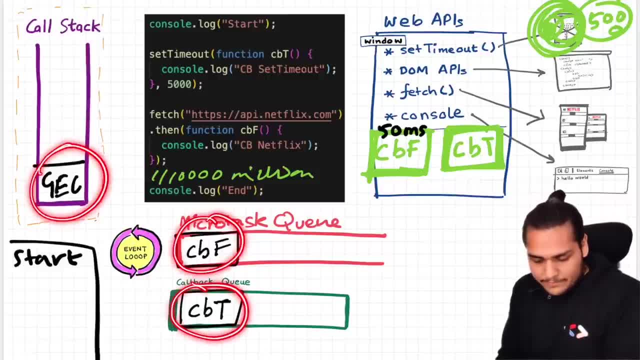 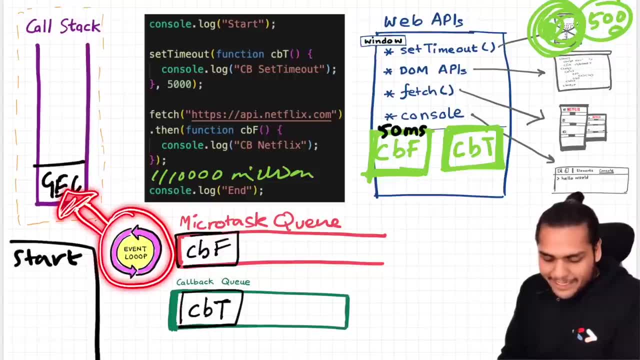 And both of these tasks are waiting to be executed and the code is still running. now the job of this event loop is to continuously check whether the call stack is empty or not, And if it is empty, then just schedule these tasks. So suppose this million line of code is finished executing now. 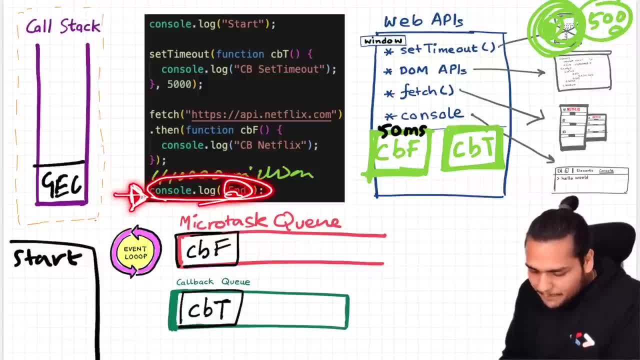 And we reach this line, console dot log end. So this end will be printed over here first. right, This end will be printed over here in the console And there is nothing else to execute now. The global execution context will be popped out of the stack. 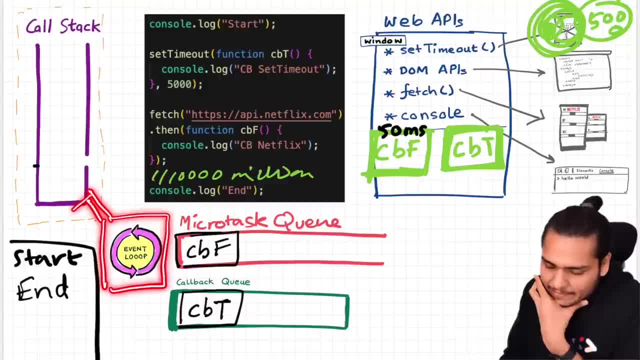 So this event loop continuously Is monitoring the call stack and once the call stack is now empty, It also sees that there are some tasks and say pending inside the micro task queue as well as the callback queue, But because this micro task queue has the higher priority, 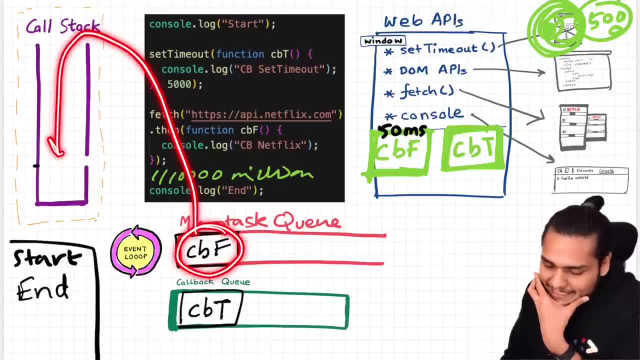 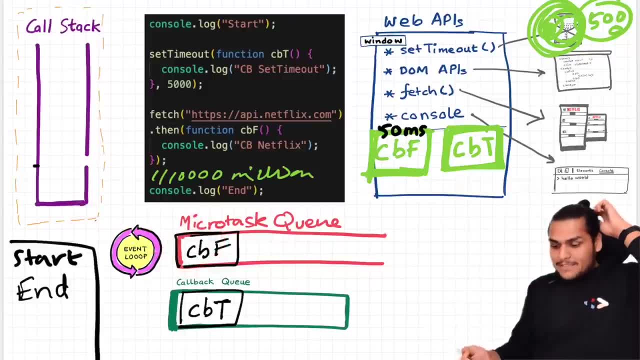 It gives the chance to the CBS function to get inside the call stack. It just take this function CBF and puts it inside the call stack. Now, again, the same history happens. this callback CBF will be pushed inside the call stack. Okay, it will get. this execution context will be there and now it will run the code of the CBF function. 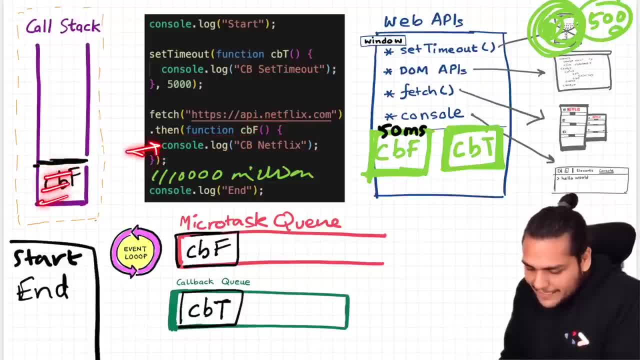 This function line by line. over here It console logs: CB Netflix right. this callback works was from Netflix right, So it prints the CB Netflix over here in the console- CB Netflix Right- and it is popped off from the call stack. It's gone. 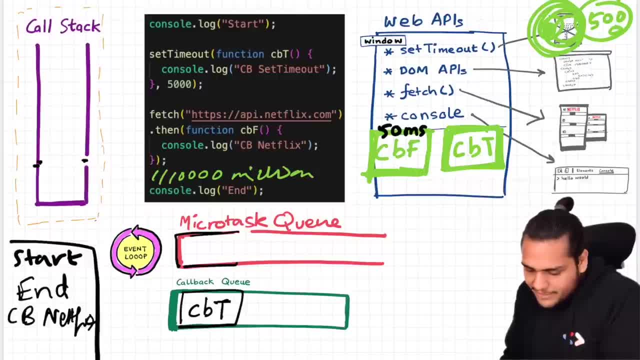 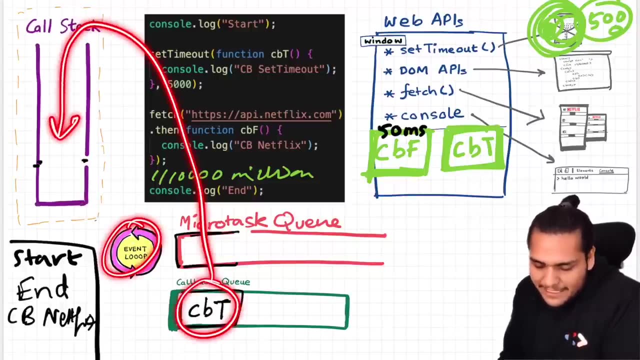 And gone from here. also, right, We should have removed it earlier. only Meanwhile all this is happening. This event loop is again monitoring, right, the call stack. as soon as that function, CBF- is like done with the job event loop, Then she deals the CBT function inside this call stack and it executes. 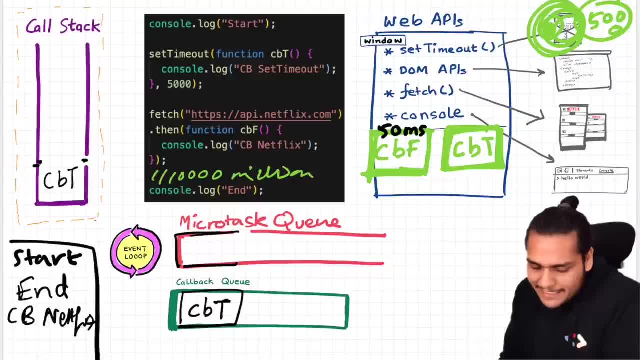 So again, the CBT function will go inside this call stack and this execution context will again run the code of the CBT function. This time the CB set timeout will be printed in the console And the whole code will be executed like this. So that is how this whole thing works. 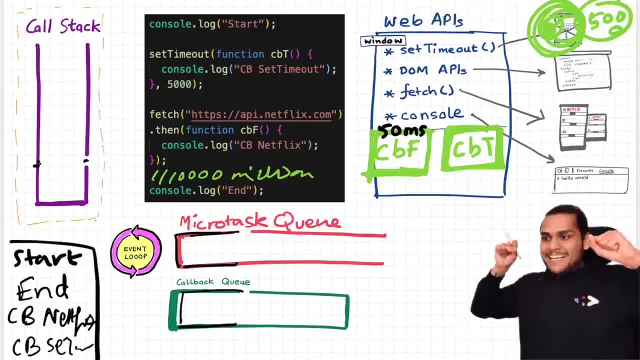 Wow, amazing, isn't it? I am tired. I don't know about you, but this is like something super amazing thing which the browser is doing behind the scenes, isn't it? So there is one last small thing. Let me cover that too. 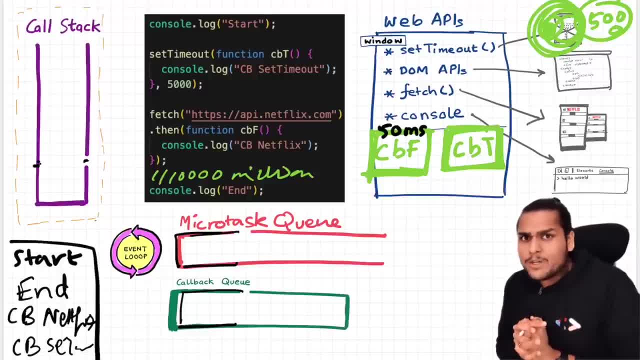 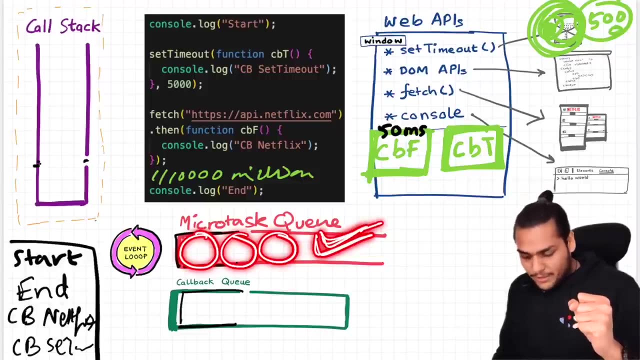 Now we have covered so much. I know you must be tired, and me Too, but let's cover that too. That is a very important interview question. Okay, so you know this micro task queue is given priority. Okay, so the question arises that what can come inside this micro task queue? 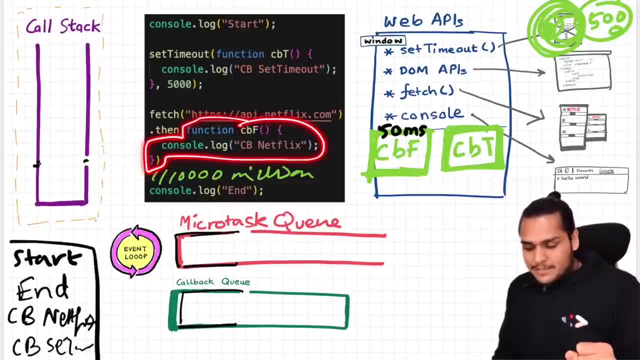 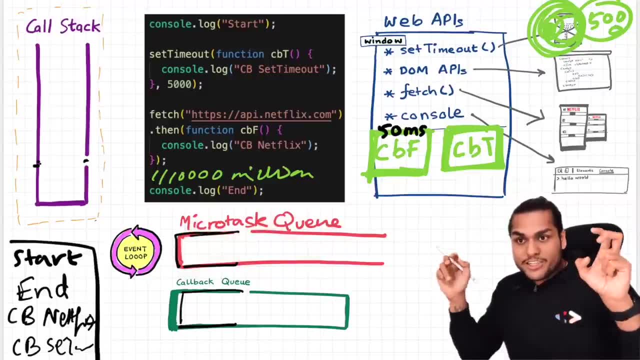 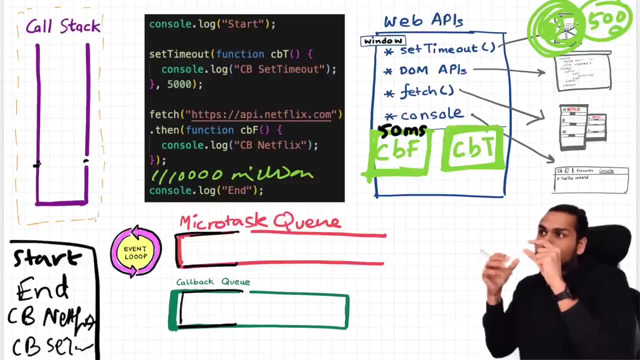 All the callback function which comes through promises will go inside this micro task queue. Okay, and there is something known as mutation observer. So mutation observer Basically keeps on checking whether there is some mutation in the dome tree or not. If there is some mutation in the dome tree, it can execute some callback function. 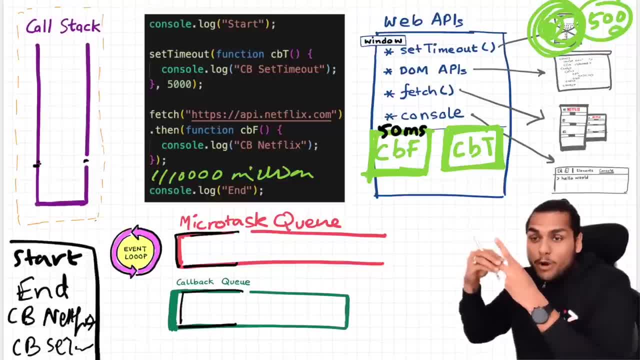 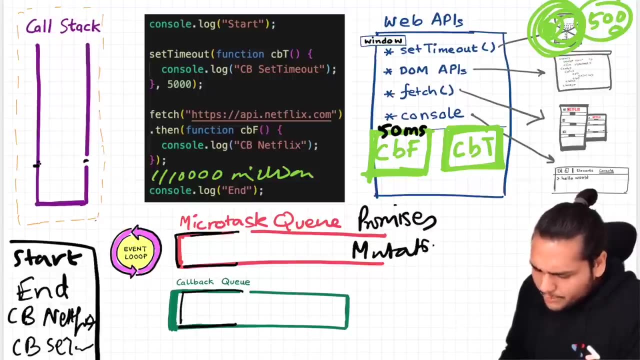 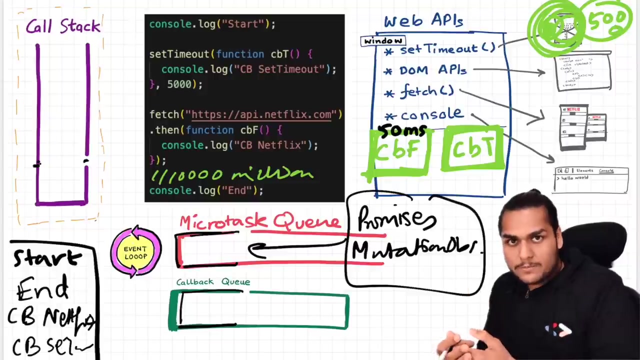 Okay, so these two things: promises, the callback function, which are which come through promises, as well as mutation observer. Let me write it down for your reference. Okay so, promises and mutation observer. You can read more about it. For sure, This is your homework- goes inside this micro task queue, but all the other callback functions, right. the callback function which comes from set time out, the callback function which is from the Dom API is like the event listeners, and all all that goes inside this callback queue. 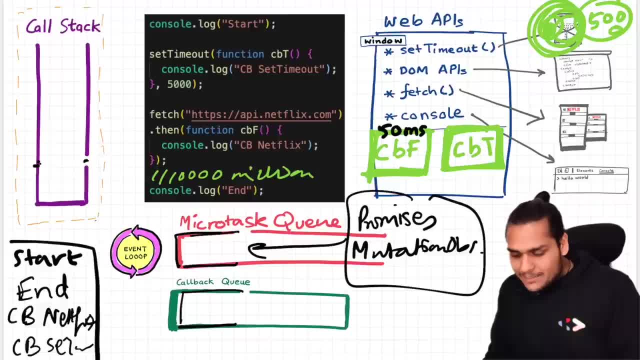 Okay, so all everything else goes inside this callback queue and these two things goes inside the micro task queue and these are given more priority. So this callback queue is also known with some fancy names like task queue. Okay, some people call this queue as task queue, right? 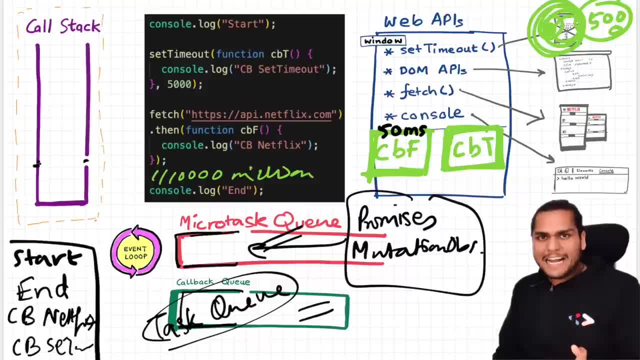 This is the task queue. This is the micro task queue. Okay, I don't call it my task queue because it is confusing, right, micro task and task sometime gets confusing. So I just call that as callback queue, right, Because it is like in general, all the callbacks come into this queue and micro task queue is the queue. 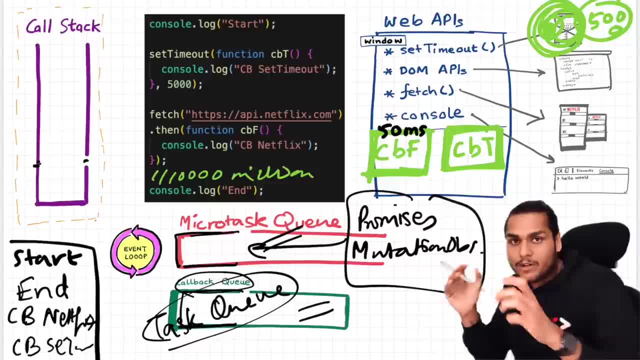 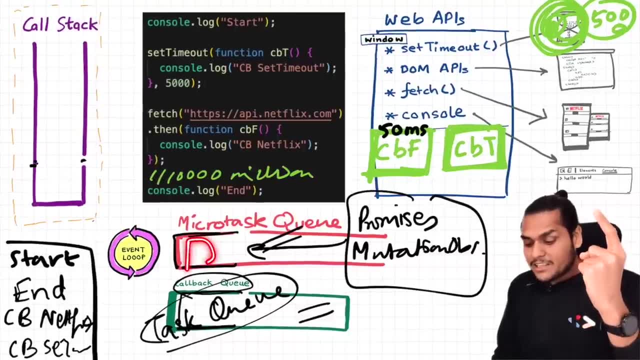 Which has the callbacks just from the promises, and mutation observer. Okay, these are the two things, and there is one more important thing to note over here is that suppose there are three micro task pending inside this micro task queue and we have one task inside this callback queue. 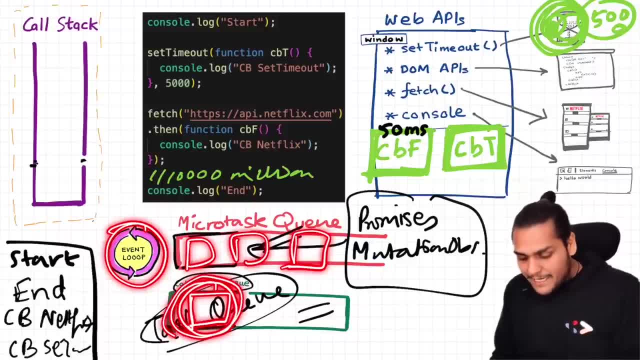 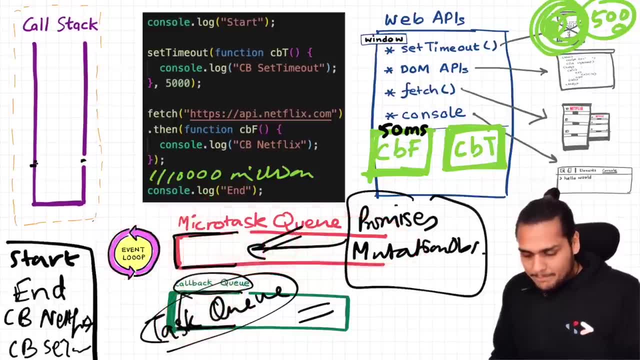 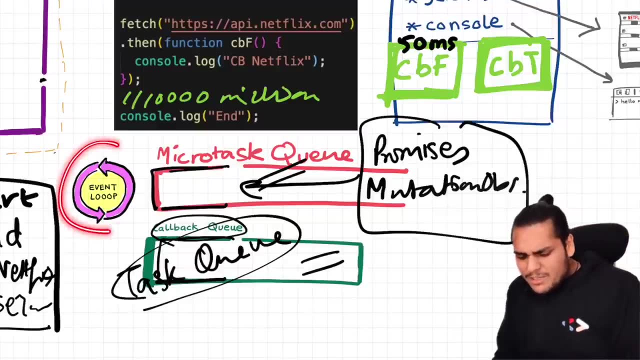 So this event loop will only give opportunity to this callback queue task once all the tasks from the micro task queue is like completed. So just one last thing- Yes, this is definitely the last one and the most important one- is that, just because this event loop gives chance to micro task first, right. 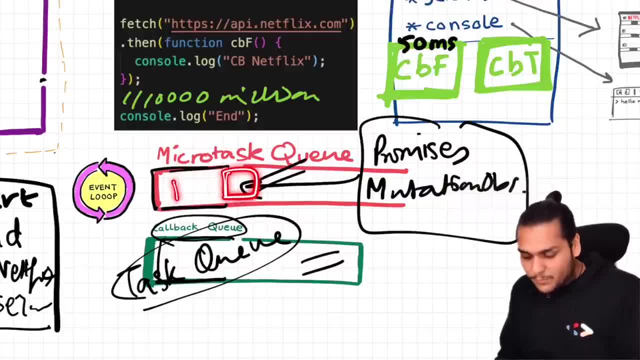 So suppose there is a micro task here, It gives us this micro task first chance before any of the callback queue task, right? So what will happen? Suppose if this micro task creates a new micro task in itself, right. If suppose this task, when executed, creates another micro task and this task creates another micro task. 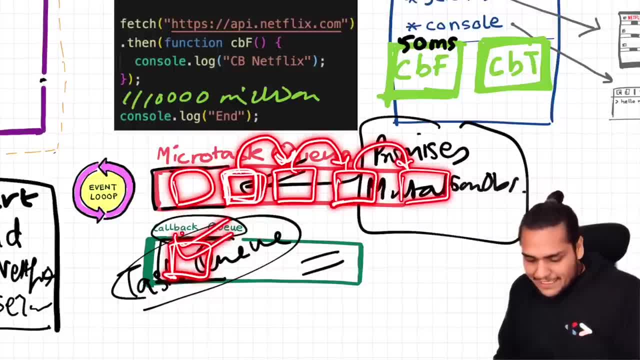 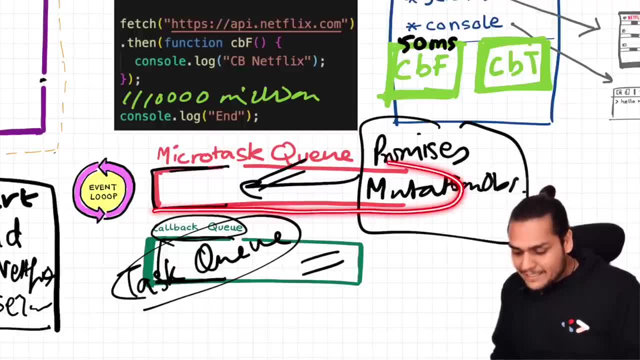 And it goes on like this. So this task over here in the callback queue will never get a chance to execute right, Because this micro task has more priority. That means there is a possibility that the task waiting over here does not get a chance to execute it like for a long time. 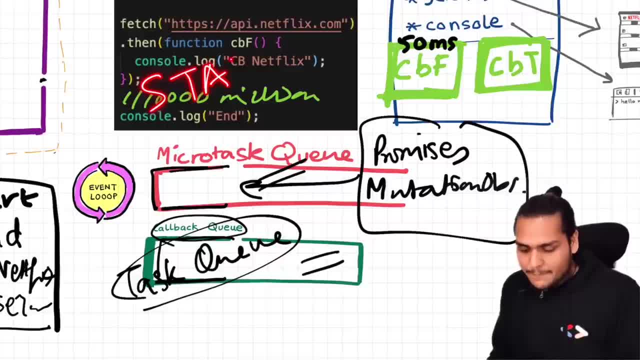 And in this case this is known as starvation- Okay, starvation of the callback queue of the task inside. This is a possibility, this can happen. So if you want to read more about this, go do some research, do some homework and you will get to know a lot of information about it. 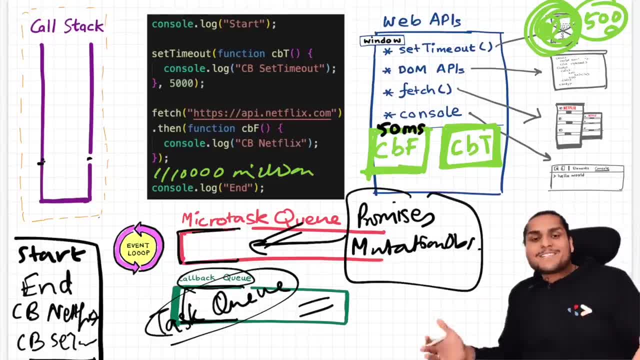 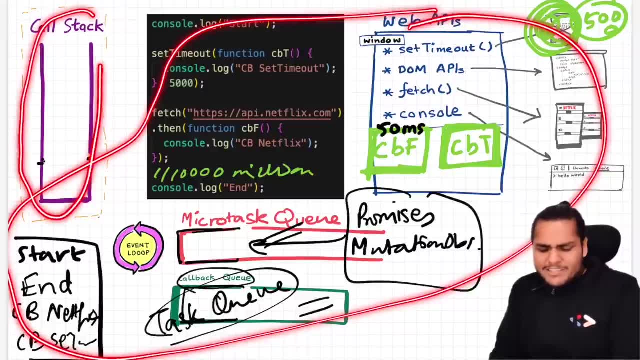 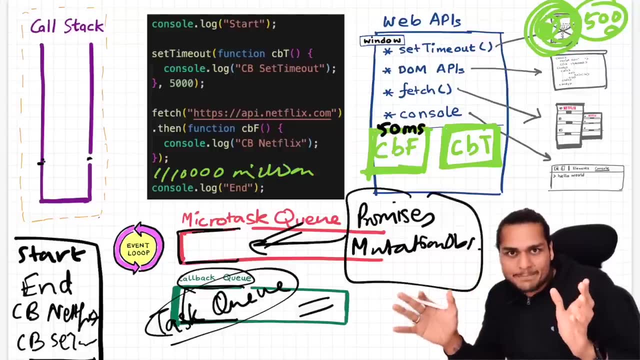 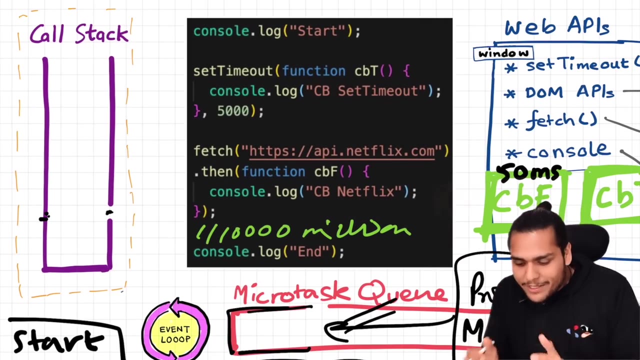 Very interesting it is. So now, my friends, you must be wondering that whatever is happening over here is happening inside the browser and JS. actually, this JavaScript engine does not do much of work, But don't underestimate JS engine. don't underestimate this JS engine. This JS engine in itself does a huge amount of work inside over here, right? 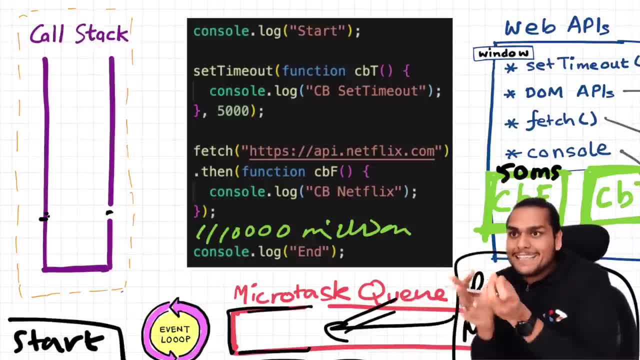 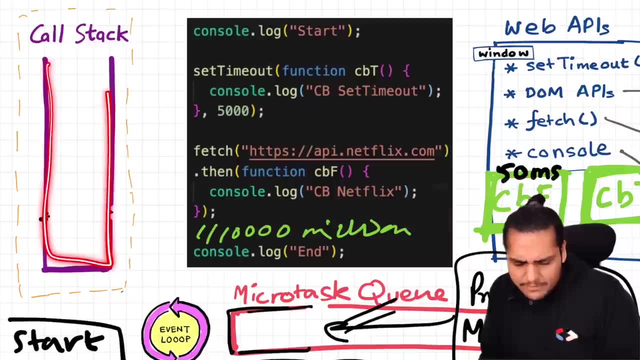 So in this video we saw the power of the browser and the web APIs. In the next video, we will see the power of the JS engine. We will dive deep into the JavaScript engine and will understand what happens inside this JavaScript engine. Is it just this call stack? 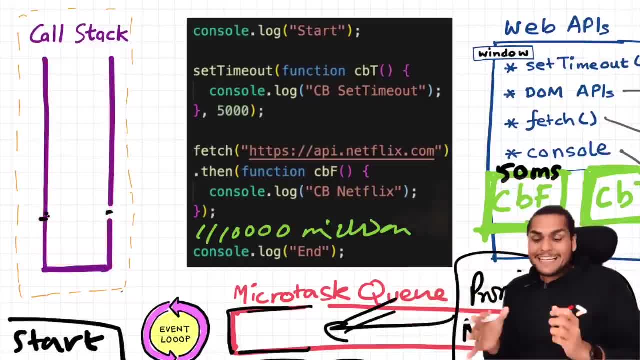 No, no, don't underestimate it. There is a lot more things With the JavaScript engine itself. We will cover in the next video the whole JS engine architecture. We will also see what is a JavaScript runtime, What is the difference between JavaScript runtime and a JavaScript engine, and how everything works and how things look inside the JavaScript engine. 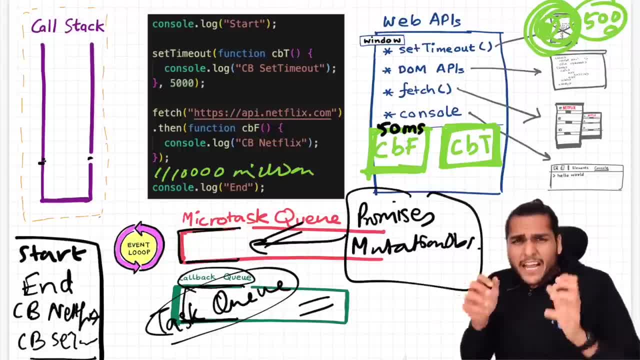 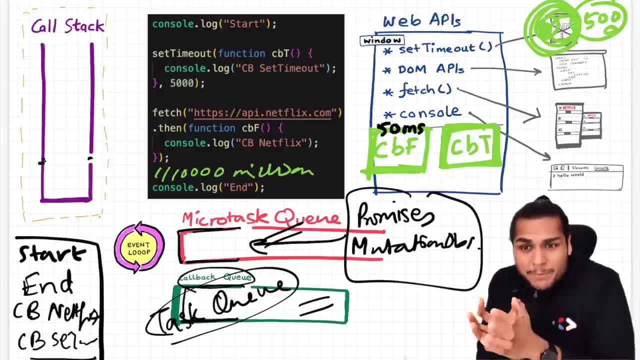 I know this is too much in a single video, but hope you have enjoyed it. I have put in a lot of efforts to create this video, So do let me know in comments whether you understood the topics or not, whether the explanation was Good or not.